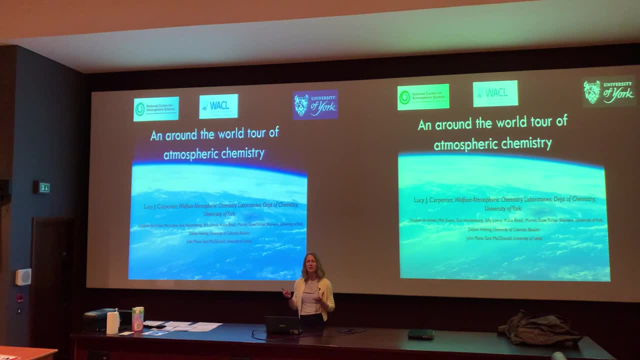 So, like a lot of science now, I work in a large team, So a lot of scientific research now is done. you know we don't really work in solo groups anymore, we work in large teams. In the Wackham Laboratory there are now around about 70 of us. 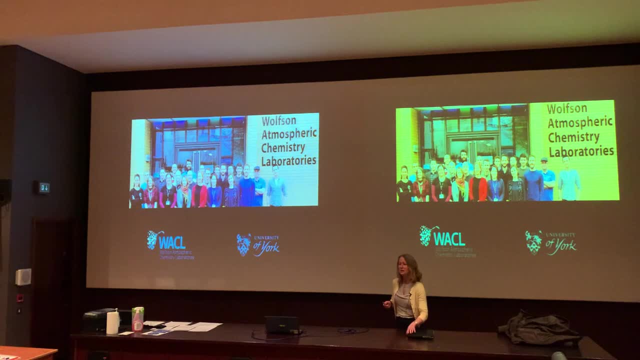 When I first arrived at York, which was over 20 years ago now, I was the only atmospheric chemist, And now there are about 70 of us. I like this photo because it looks like I'm the boss. I'm sat in the middle there. 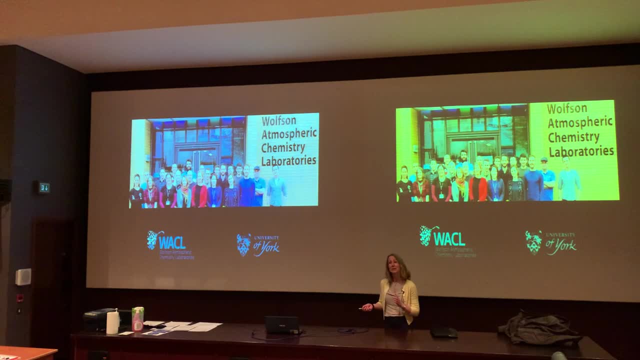 I'm not in charge. no one's really in charge. well, no one knows who is in charge, but it seems to work quite well, And along with around seven academics, there are about 60 PhD students, postdocs and technical staff as well, from a range of backgrounds. 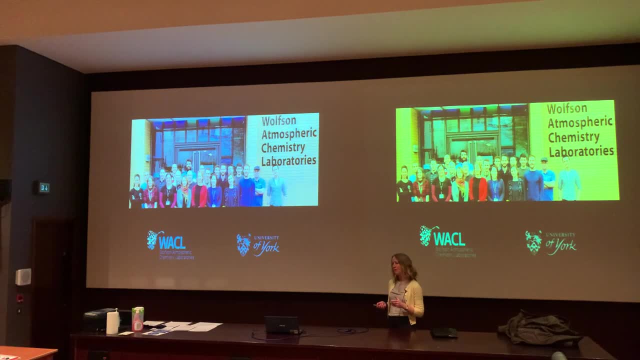 We sit within the chemistry department at York, so we have a lot of chemistry PhD students or graduates, chemical graduates, but people with environmental science background. We have backgrounds in physics as well, and more and more we work with big data and in data science. 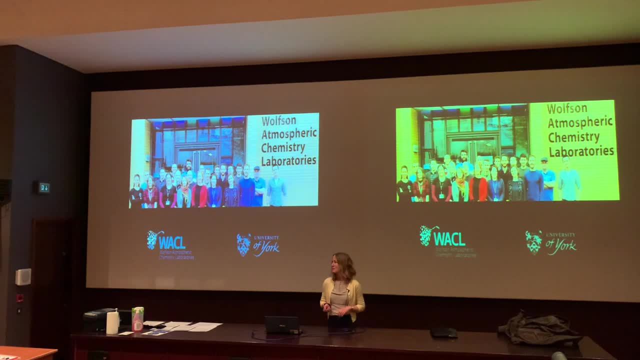 We're finding students with computer skills are very useful to us as well. So that's the background that we have And, as I said, I'm an experimental atmospheric chemist And a lot of what we do involves going on fieldwork measuring different molecules in different parts of the world. 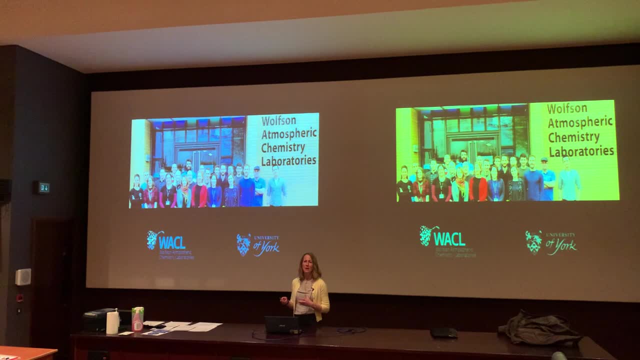 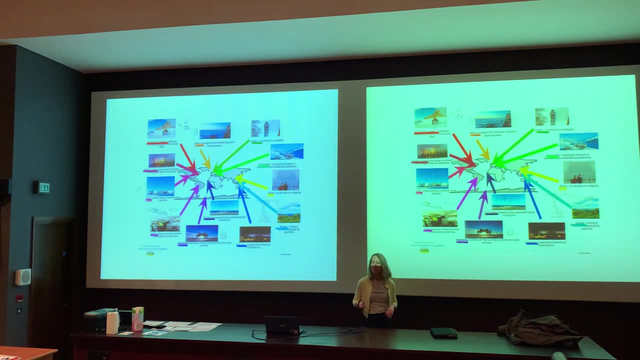 and really making discoveries about what's driving the atmospheric chemistry in most parts of the world. So this is just an example of some of the places we've migrated into over the last 10 to 15 years, And I don't know how well you can see this, but this is a sort of cartoon map of the world. 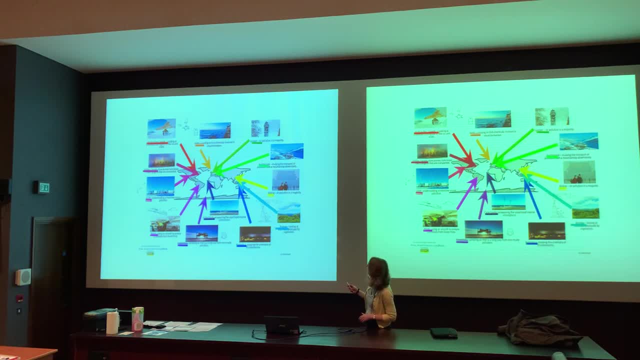 We have done field campaigns in very polluted regions. So, for example, when we're studying air pollution, there's been some campaigns in Beijing looking at air pollution. in the big city There is continuous monitoring going on on the beach. We're going on the BT Tower in London. 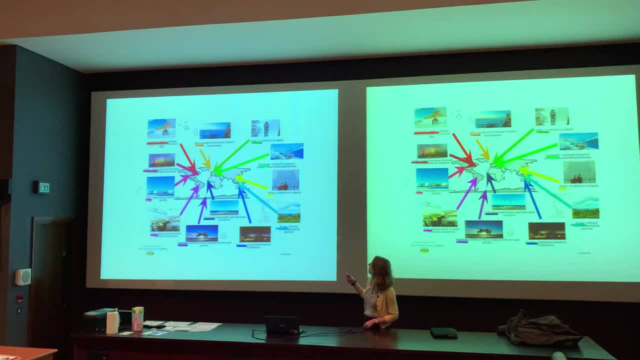 If you've ever seen the BT Tower, you look up there. there's monitoring equipment owned by various universities around the UK, including York, where we can pick up pollution there. There have been various campaigns in places like Canada and in Brazil as well. 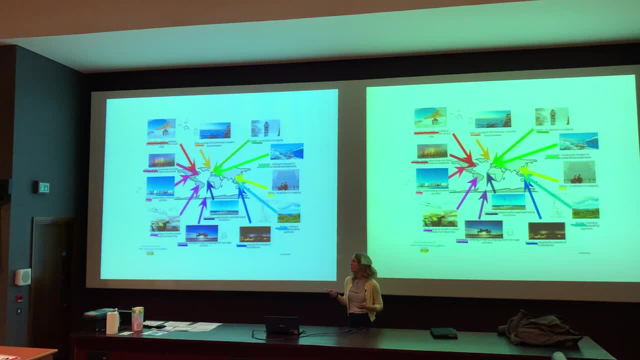 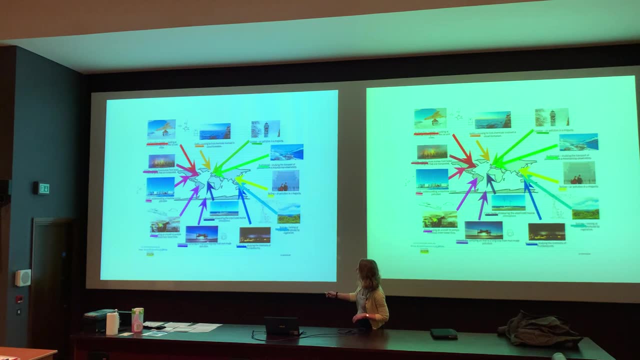 looking at forest fires and the sort of chemistry that happens over forest fires Or, for a complete contrast, places like Antarctica. I don't know if you can see. this is in Halley in Antarctica. there's a big station sitting there above the ice. 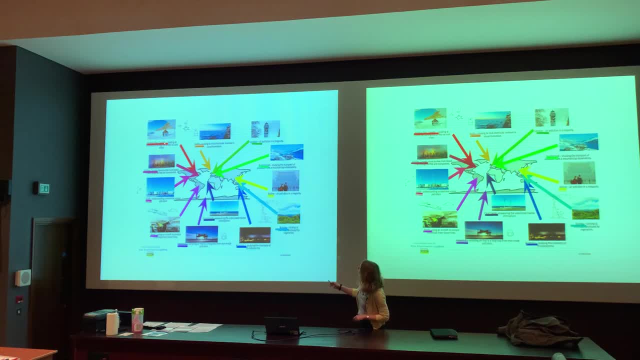 looking at really, really remote chemistry And similarly in the Arctic, where we've been on ships that basically are icebreakers. go through the ice and look at special chemistry that happens on ice that might contribute to what's going on in the atmosphere. 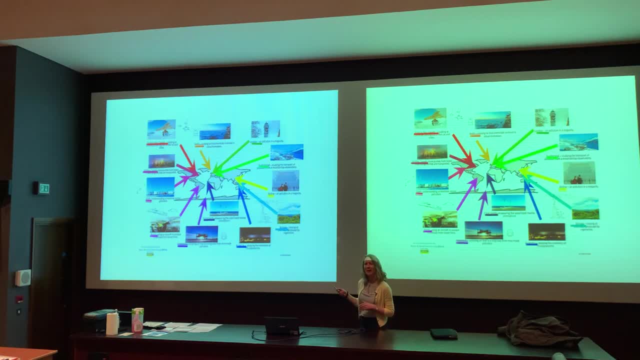 So you kind of think: well, the life of an atmosphere chemistry doesn't look bad flying around the world, but do you really need to do that? Obviously, now we have to have an eye on sustainability. We don't want to be creating the problems that we're also trying to solve, in a way. 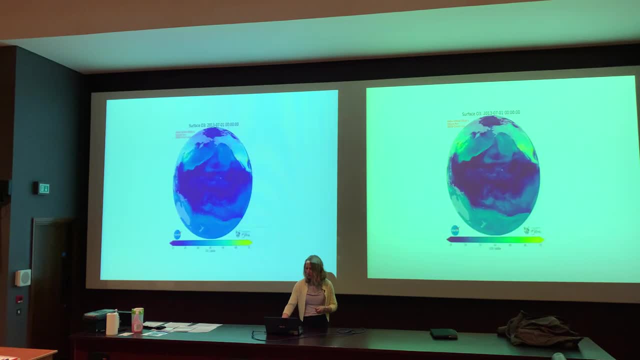 So I'm just going to try to demonstrate to you why we have to, in a way, go to various places around the world to discover the atmospheric chemistry that they have. This is just a movie, if it works- of the 3D model of tropospheric ozone. 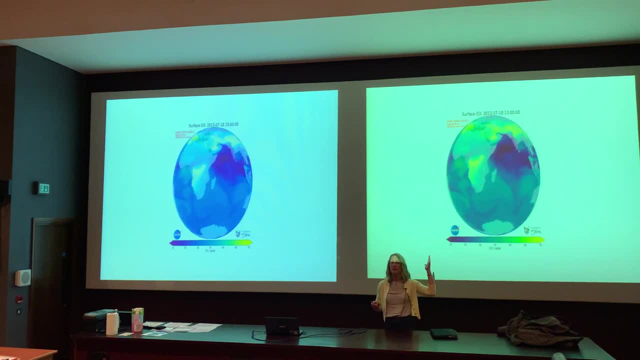 So this is ozone in the surface. This is the surface layer of the atmosphere, So not stratospheric ozone which is 10 to 20 kilometres high, but the stuff at the surface which we breathe in, And I'll show you why that's important a little bit later. 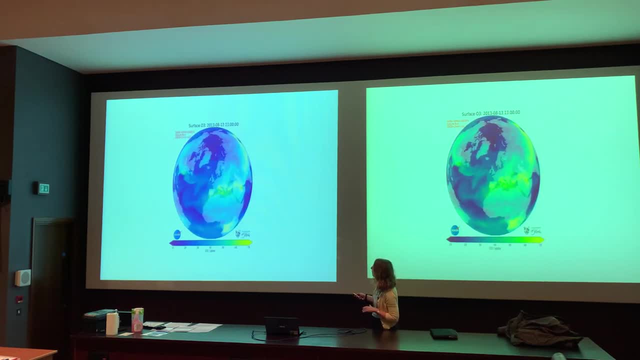 But as this globe kind of comes round, the warmer colours, the yellow is the higher ozone You can see it pulsing. That's different because ozone has a cycle, that it pulses by season and it goes up and down during the day. 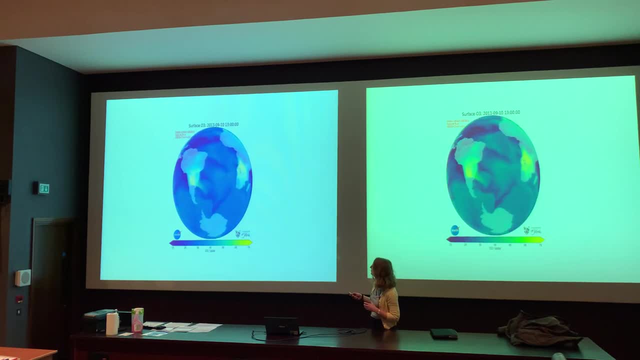 But it has very, very different characteristics in different parts of the world. So when you see, for example, it going over South America, which we'll see in a moment, there are large biogenic sources from forests, So it's a very rich mixture of hydrocarbons that come from here we go. 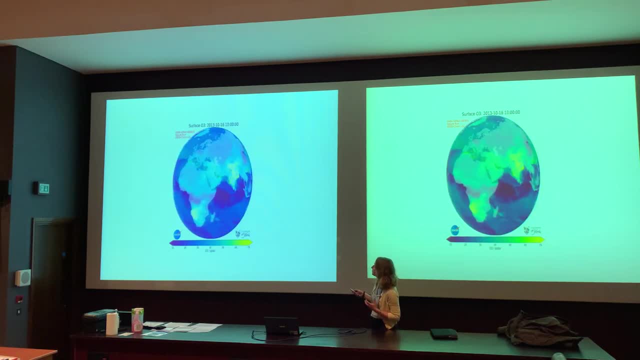 there was just Brazil that went past just there. Those sorts of forest regions you know you'd find in some parts of the world but not in others. There's special chemistry happening over the ocean that we need to take a look at, And so there were different processes happening in different parts of the world. 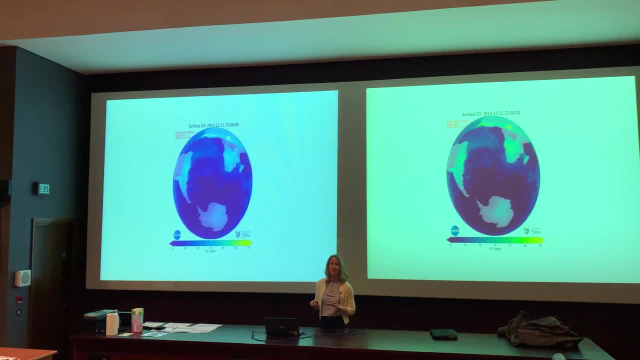 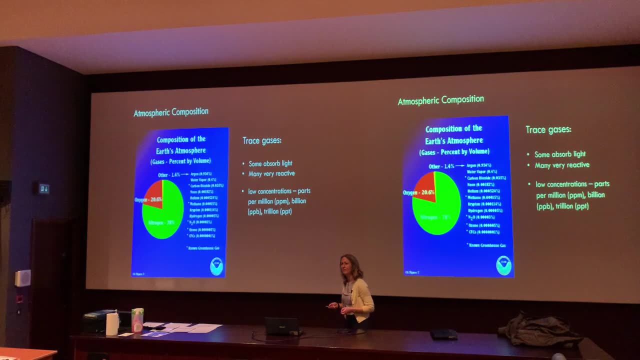 So there were different processes happening in different parts of the world. So there were different processes happening in different parts of the world that you can only really discover by going there and that you might only observe by travelling there. So that's kind of the excuse, if you like, for why it does involve a lot of fieldwork. 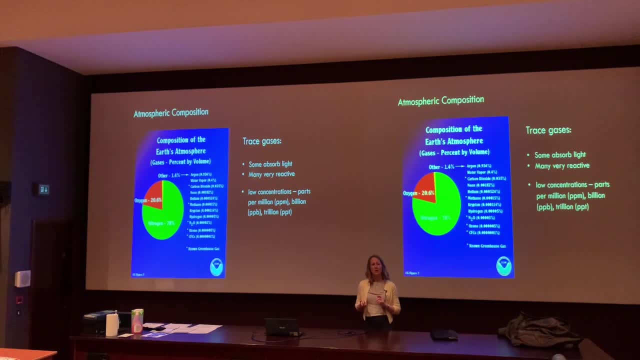 This slide gives you an idea of the challenge that we have. You probably know that most of the atmosphere- so around about 99% of the atmosphere- is made up of oxygen and nitrogen. So obviously, nitrogen around 80%, oxygen around 20%. 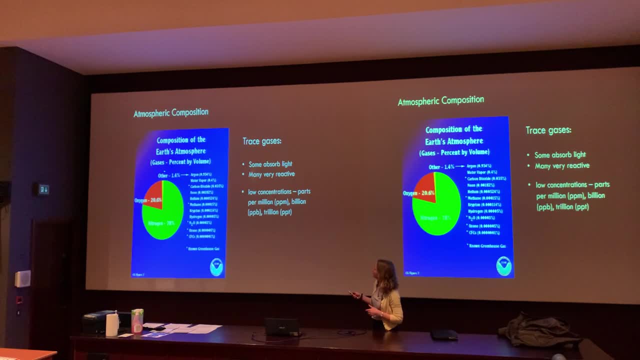 So all of the other gases only make up oxygen. So we can only make up around about 1% or so, And almost all of that 1% are gases that, as a chemist, I have no interest in. So I don't really care about the noble gases. 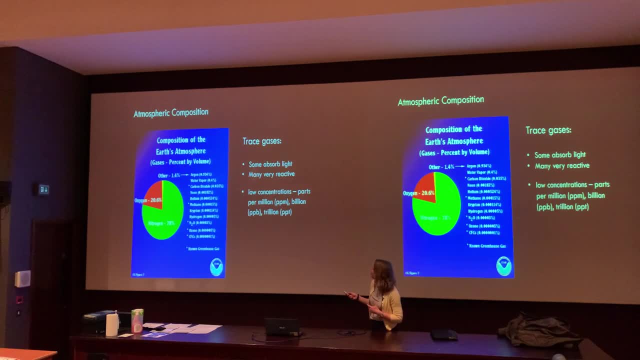 They have no chemistry, They're not doing anything interesting for me. And even CO2,. obviously we know CO2 is a greenhouse gas, but actually it really doesn't have any atmospheric chemistry. The science around CO2, and understanding how it's taken up into the ocean. 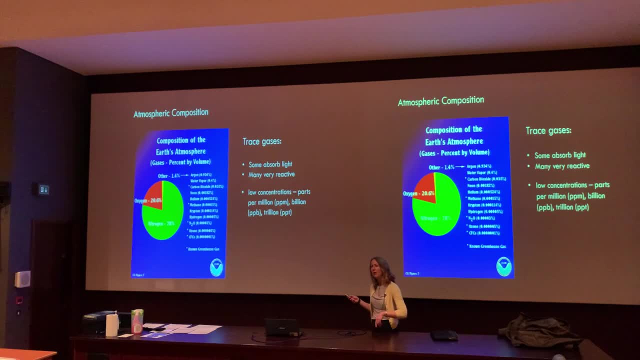 and how it's cycled in the ocean, how it's cycled through the carbon cycle and creates global warming, but it's not really a sort of chemistry molecule, if you like. You have to really get down to these very, very low percentages. 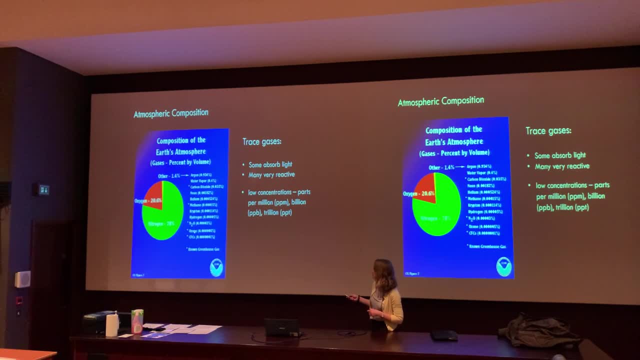 until you get to gases that have chemistry, So gases like ozone, for example. many, many fractions of a percent, In fact. we mostly express them in units of these mixing ratios here, so parts per million, parts per billion, parts per trillion. The reason, of course, they are so low in concentration is because they are reactive. So if you're reacting with lots of other gases, the concentration is kept very low. But even though these gases are very small in abundance, they punch well above their weight in terms of the impact that they have on the atmosphere. 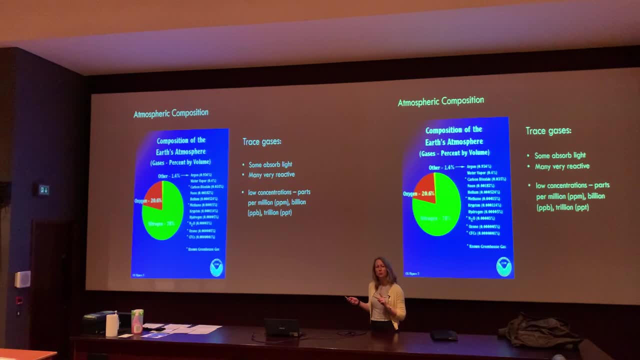 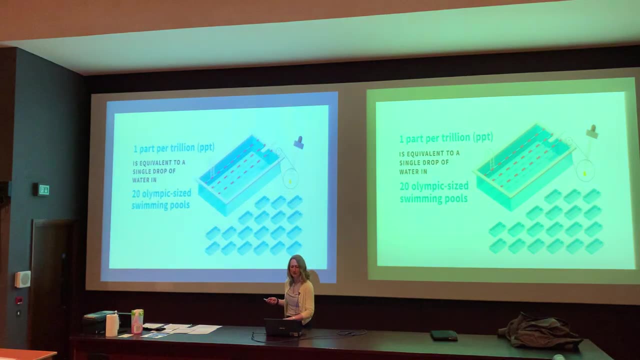 And so a part per trillion means there's one molecule in 10 to the 12 other molecules, And so, to give you an idea of what that looks like, trying to measure that in the atmosphere, that's the same as one drop of water in 20 Olympic-sized swimming pools. 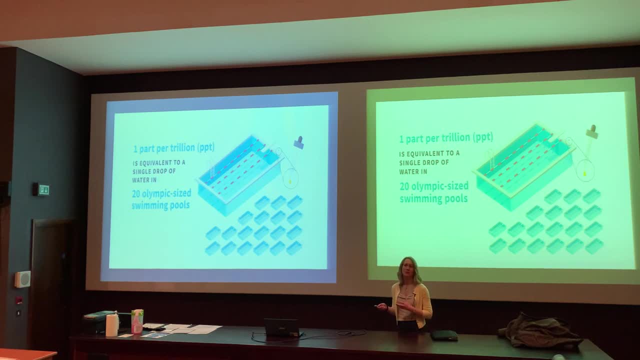 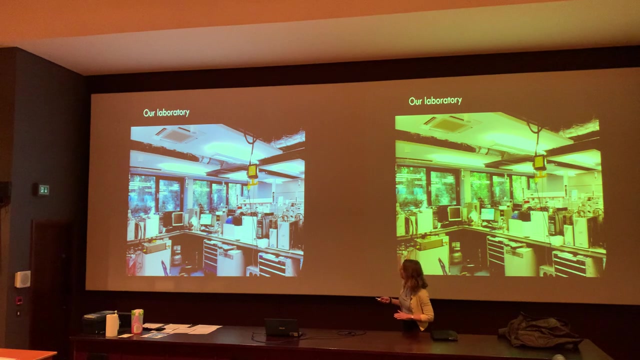 So that's the level of challenge, if you like- that the instruments that we use have got to try to really sniff out those tiny concentrations and to be able to measure them accurately and precisely. So this just shows a picture of one of our labs in the WACO building. 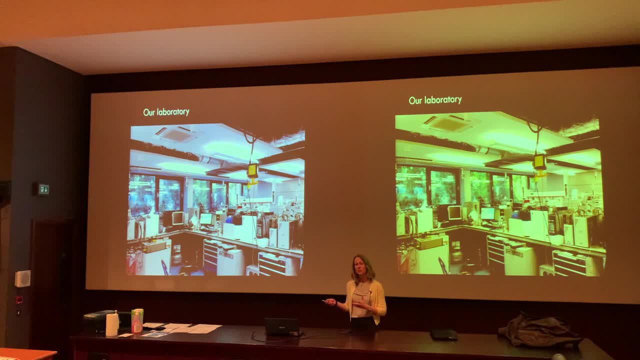 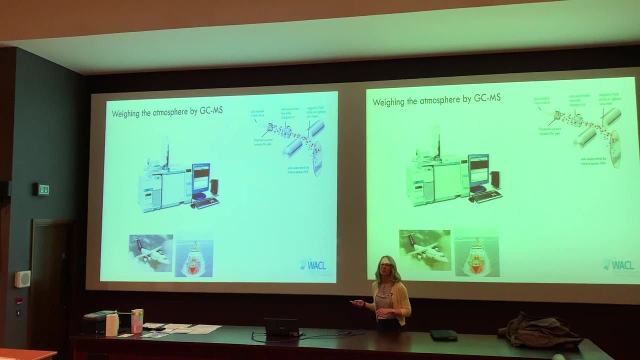 And we have these big shared laboratories, which is great. People can swap and share equipment And we use a sort of mixture, I suppose, of commercial instrumentation and instrumentation that we've built ourselves, And sometimes we take commercial instrumentation and then adapt it to what we want to do. 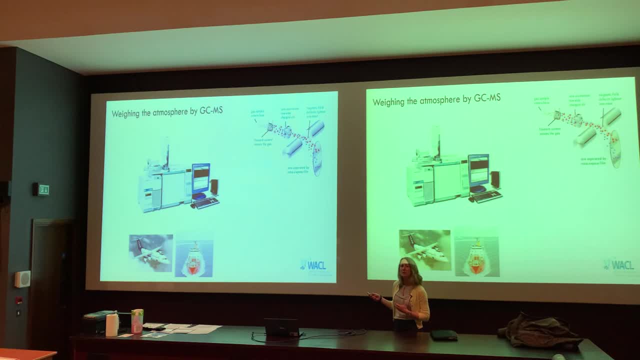 So this is just a straightforward GCMS. You may have used this in some labs. I don't know if you've done a bit of it in your chemistry labs. It's a well-established technique that essentially ionises gas molecules and separates them. 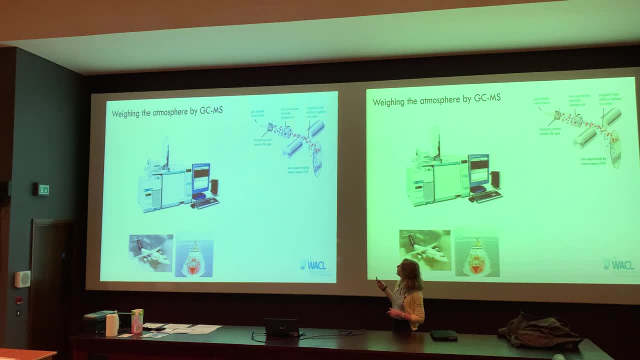 It separates them according to their natural charge ratio by accelerating them through various fields. So you can find these off the shelf, of course, And they've got better and better as the years have gone by. But so for various of our applications, we can't just take them as they are. 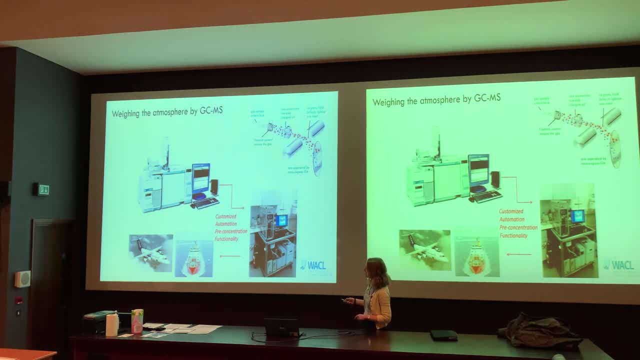 So, for example, some of what we do involves measuring gases in seawater on board with search cruisers. So we have to this. you can't really see it very well. It's not the resolution's not great, but this device here essentially. 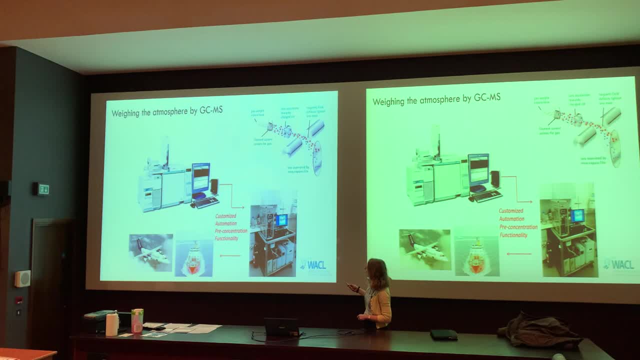 we can pump the seawater through here. It strips the gases out that we want to measure Those gases. now they go down into some units down here which we fill, which enable those gases to be pre to be concentrated up. So we get rid of the gases. we're not interested in: the oxygen, the nitrogen, the CO2.. 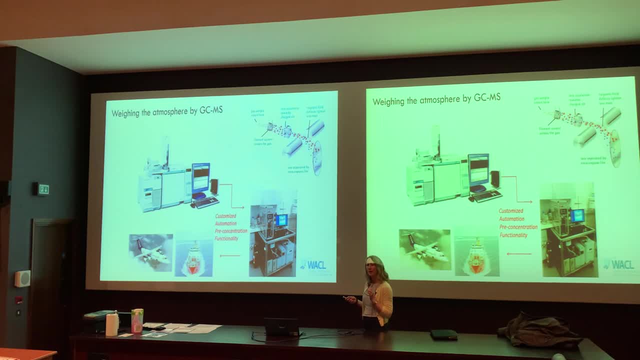 And you're just left behind with the ones you want to measure, And that enables the sensitivity of your equipment to be way, way higher than it would be otherwise. So that's one way we do things. There's all sorts of different ways we can do things. 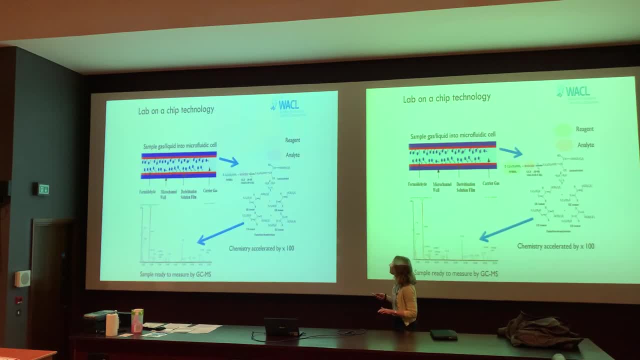 We can pump the seawater through here. There's all sorts of different techniques, And this is just another example where sometimes even doing that isn't enough. So there are some gases if you, for example, are not amenable to GC or MS. 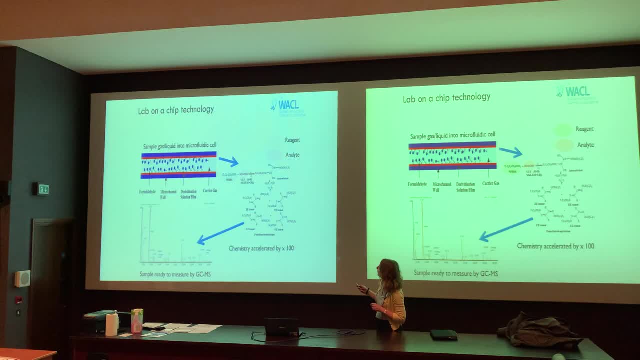 And this is an example of some- an oxygenated gaseous compound called glyoxyl And we can't put that through a GC column, so we have to react it, or with a with a different chemical to get something in the end that's stable and is quite selective. 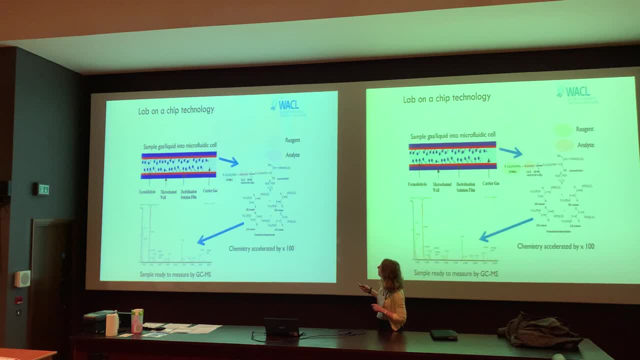 So this molecule here we're reacting in, it's got five fluorines in there And you end up with quite some stable molecules that you can then measure And rather than sort of just mix these chemicals up in a beaker or whatever and then pour them. 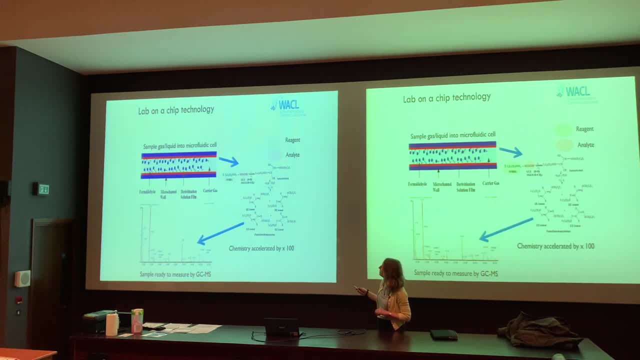 into the GC and S, we can set up sort of a clever lab on a chip technology where all of this chemistry is happening very efficiently and in an automated way before, So we don't have to do it manually, So we can accelerate that chemistry. 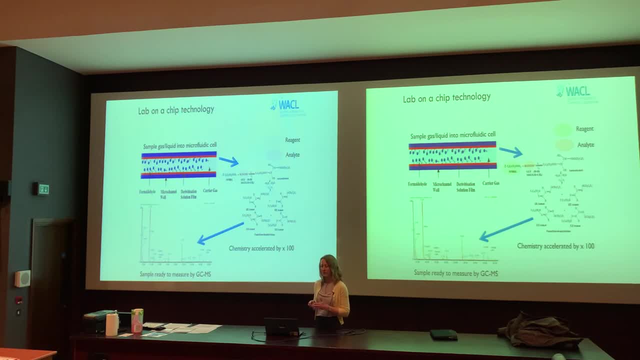 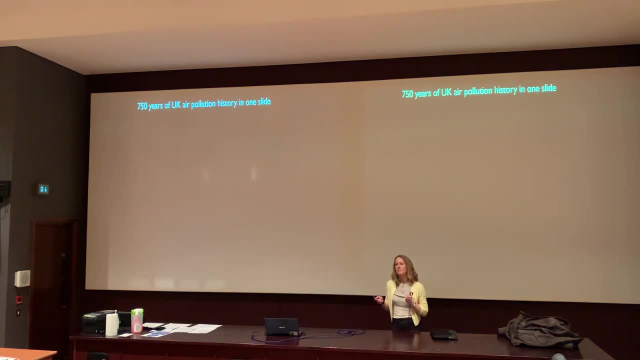 So all of this is to really improve the sensitivity And improve the selectivity of of what we do. So before I really get started on the research that we're doing in our lab, I wanted to give you a little bit of history of of air pollution. 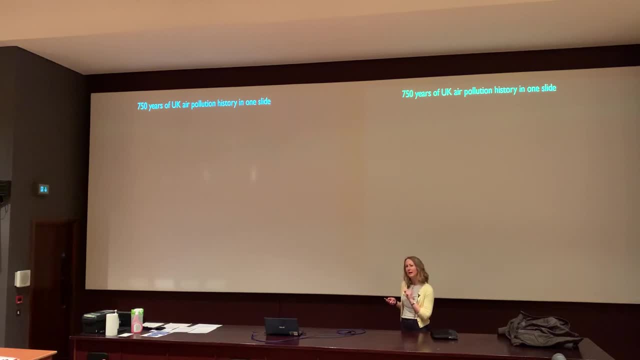 And this is going to be based pretty much on UK air pollution And really showing you 750 years of of of that history in one slide. And it starts with Edward I, who was born, yeah, almost 750 years ago. 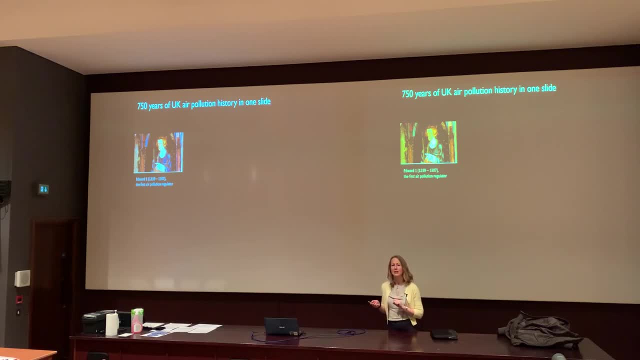 Who we consider to be the first regulator of air pollution in the UK And what he did actually. he regulated the burning of sea coal. So sea coal was when coal was brought from Newcastle to London on barges And was often. often any surface was burned very, very fine with sulphur. 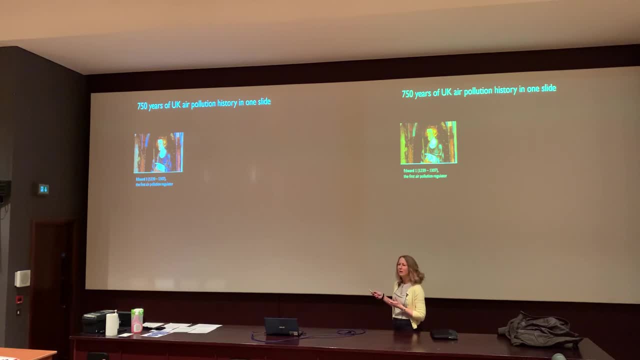 So that gave rise to pollution And he realised- or some of us who realised that you know- that that was a form of pollution. It was bad for people And so he banned it. And this is when regulators really did have teeth. 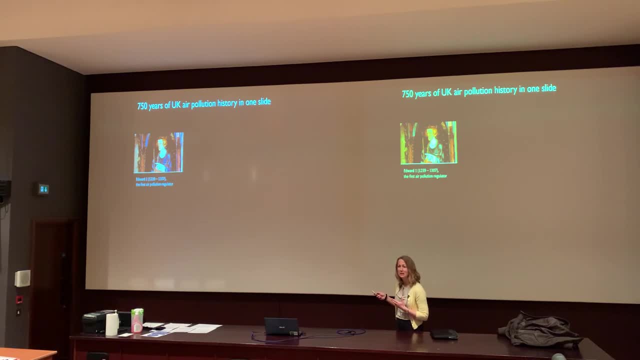 Because he actually put two people to death by full full of burning of sea coal. So so he he's considered the first regulator We're talking about 500 years later before we can trace the first person who linked air pollution with health. 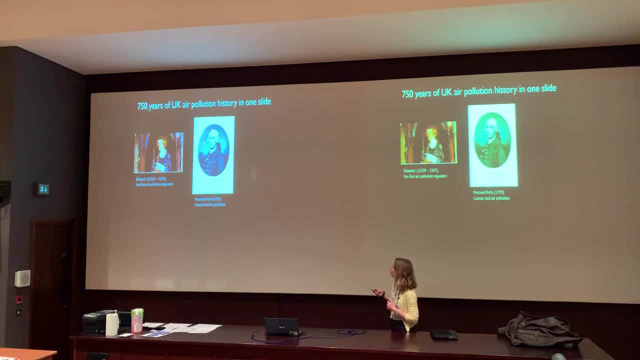 And this is a guy called Percival Potts in the mid-18th century And that link was actually between chimney sweeps and testicular cancer And that link was true. The carcinogenic PAHs, polyaromatic hydrocarbons that are in soot and in coal. 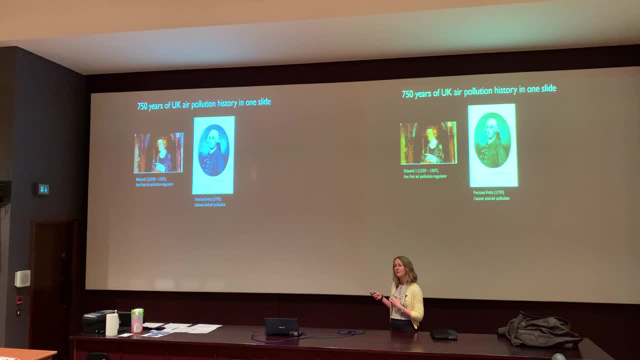 And in his notes he actually makes reference to the fact that some of these PAHs could also get out into the air. So he made that link between air pollution and health. So we have him to thank for that. In the mid-19th century you start to see the concept of air pollution occurring in the media. 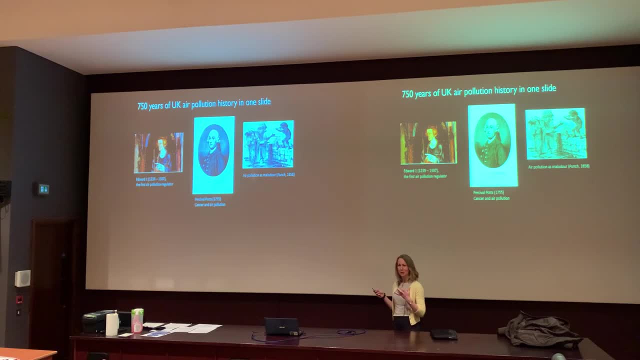 But it's mainly the concept, is true, It's essentially the smell of air pollution, So that seems to be the thing that's offending them, rather than the fact that it might be killing them as well, But nevertheless, that's what gets into the press at that point. 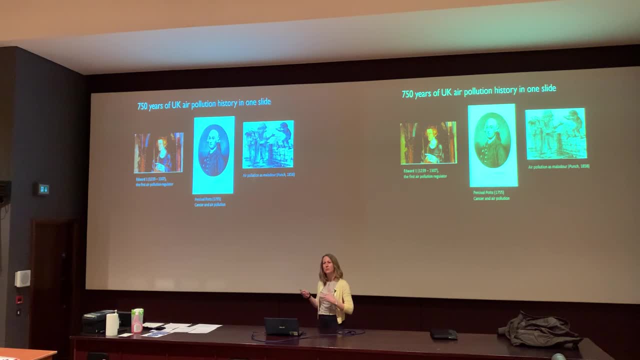 And growing awareness as the industrial revolution kicks off. I suppose that there were some downsides to this as well. And then, of course, the classic smog episodes of London in the 1950s. We start to see photographs now showing very clearly that we've got these smog episodes. I'm going to come back to that a little bit later. And then we get into the various issues of air pollution as we start to become better at measuring the air and understanding what the issues are. Acid rain was a big issue throughout, you know, particularly throughout the Northern Hemisphere, but also in parts of the Southern Hemisphere in the 60s and 70s. 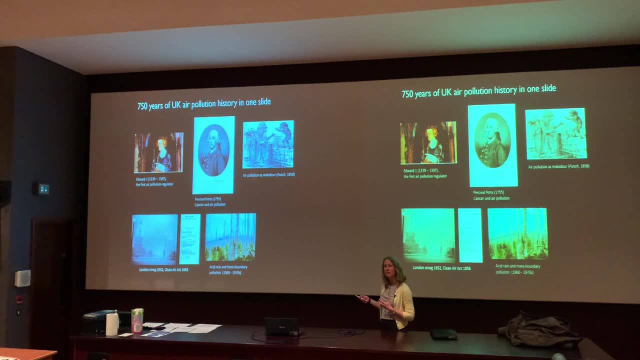 Due to a very high amount of sulphur, which is again re-promoted through coal burning, leading to sulfuric acid forming in the atmosphere, which gets into precipitation and falls and has absolutely devastating impacts effects on forests and other ecosystems as well. Now, that's a problem that we've largely 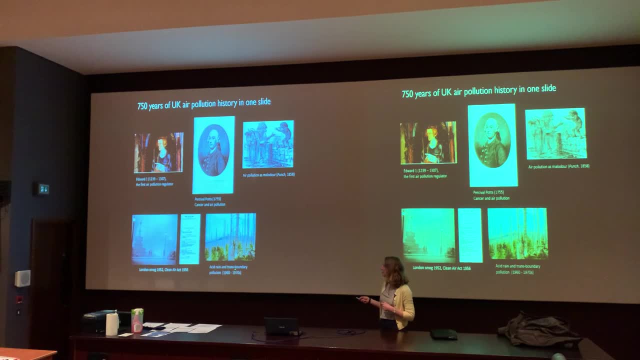 got rid of very effectively, and the reason for that is because, once it was recognised that coal burning power stations were the problem, you can remove sulphur dioxide- SO2, from the flue gas chimneys and, of course, we burn a lot less coal than we used to, as 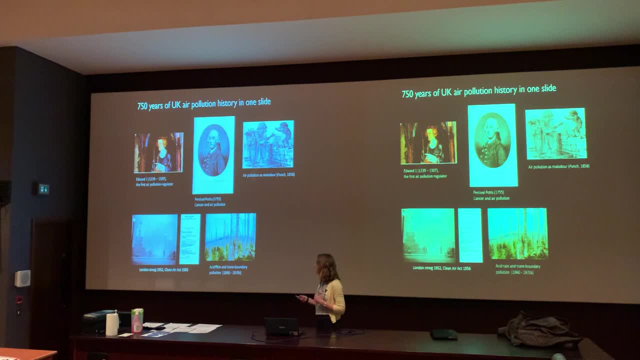 well. So the combination of those things basically means that certainly for most countries, most developed countries, we don't have this problem anymore. And then, of course, my last little bit here is the more recent scandal of Dieselgate, which I'm sure most of you were aware of. 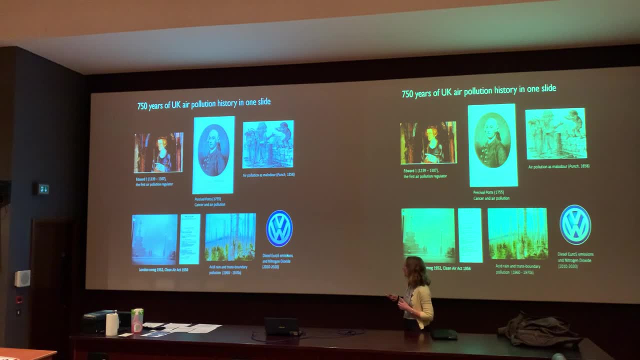 and this is really around nitrogen dioxide- And I'll come back to this later- but the fact, of course, that cars on the road were emitting way more nitrogen dioxide- which is quite harmful pollutant- than they were supposed to, and that they were measured to. 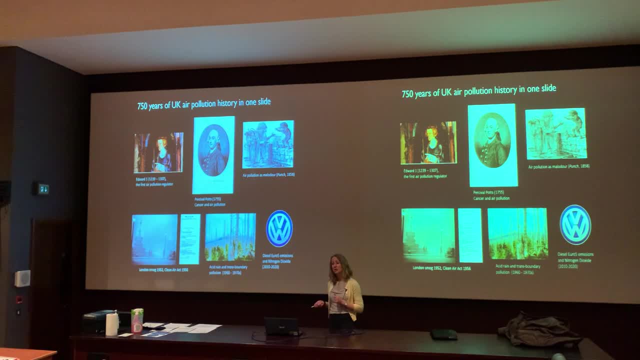 do when they would go to an NOC. So this is a quick history of, and much more has been going on in the last 50 or 100 years, I suppose, than before, But it's been around for a long time and there's a recognition. 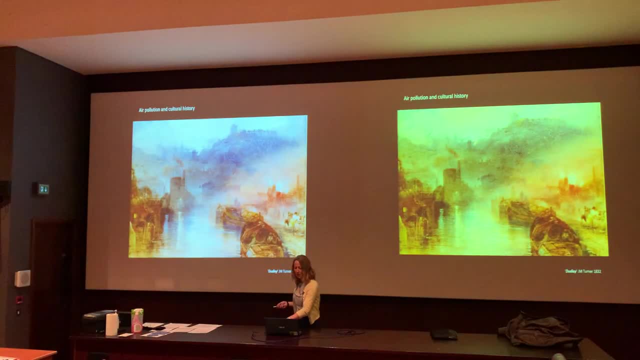 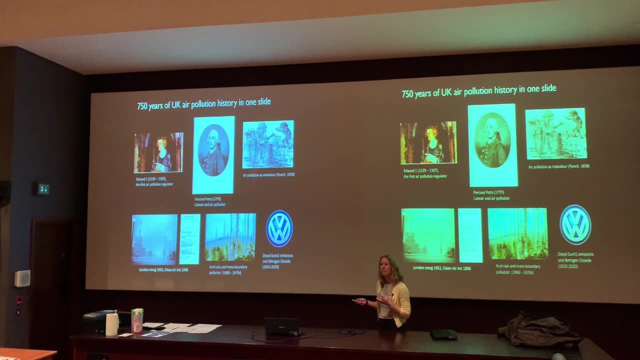 of these issues over a long time as well. Well, just before we get to that one. so I guess what is interesting is that if you look at gas like CO2, so carbon dioxide is fairly stable- we can go back nearly a million years. 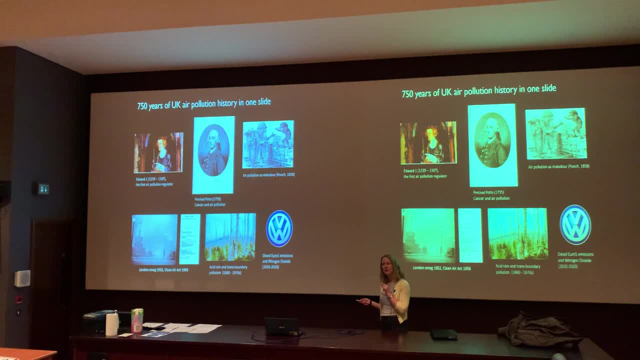 to history for our CO2 record, and that's because CO2 is very stable and it's trapped in the bubbles that you get in ice cores, So ice cores can be extracted from polar regions. you can bring that back up, measure that CO2, and go back a fantastically long time. That. 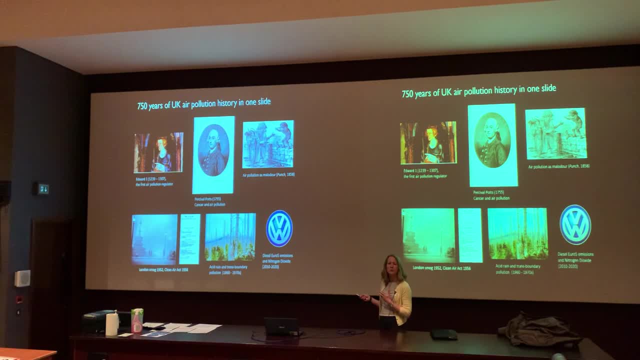 is not the case for many pollutants: SO2, or NO2, or ozone. these are all quite reactive gases. You can't simply do that in an ice core. So we don't really have very good records of atmospheric measurements- until a record. 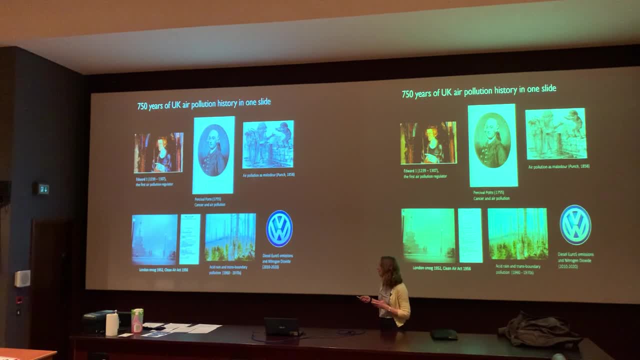 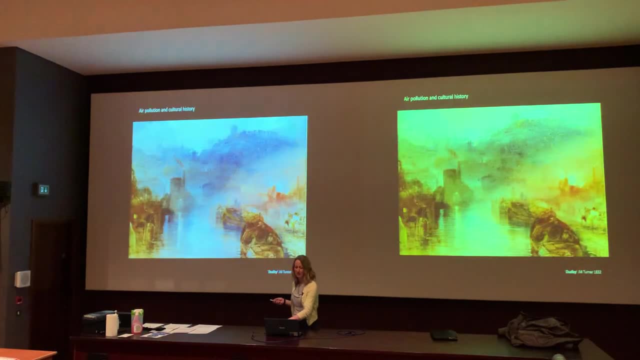 So what's interesting is that if you go back to the 1970s or so- so how do we know what we've got? if we want to go back 200 years? Look interesting. there is some evidence through art. If you go back through iconic Turner paintings, you can see a real image. 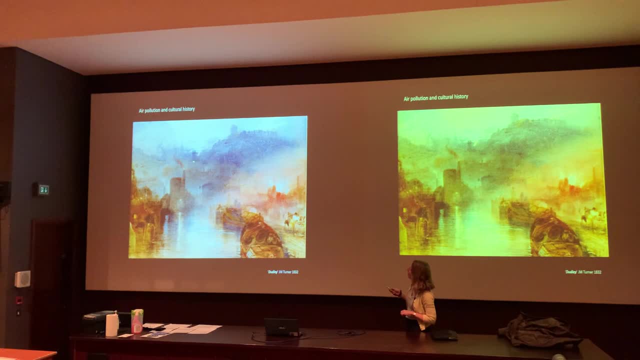 of the industrial activity that was going on and the sort of smoke-filled air that was in places like London at this time, where you've got coal burning going on, you've got domestic fires going on- All of this creating this sort of rich atmosphere of you know you don't want to really be. 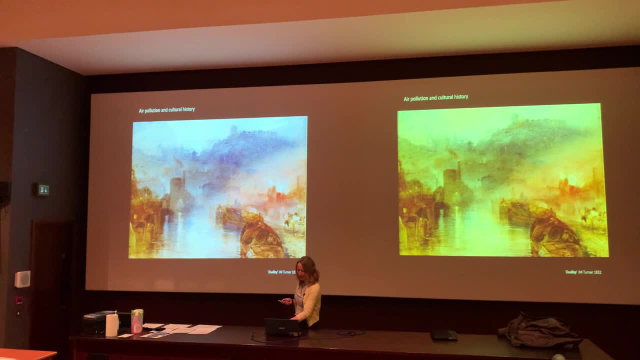 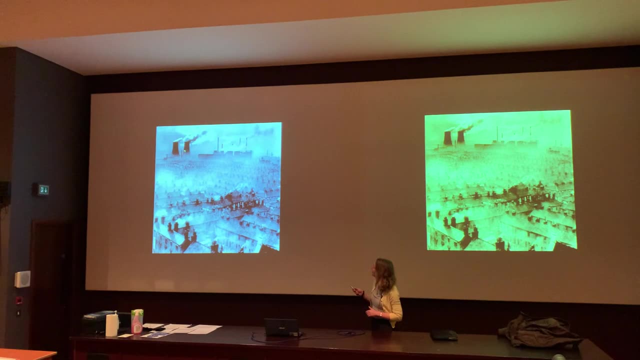 there in this picture you can see that it's going to be bad for your health. And, of course, a bit later we start to see in the 50s, we start to see actual photographs as well. This is London, of course, a fascinating power station and a typical picture of many cities. 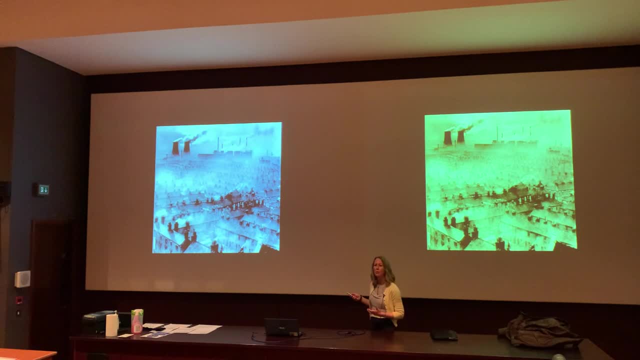 where domestic burning may be. you burn coal in an open fire in your own home, So there was a lot of pollution going on there. So this is clearly this is very much not a recent problem. The pollution at this level in these years were a lot worse than it is now in the UK And in the 1930s or so, scientists 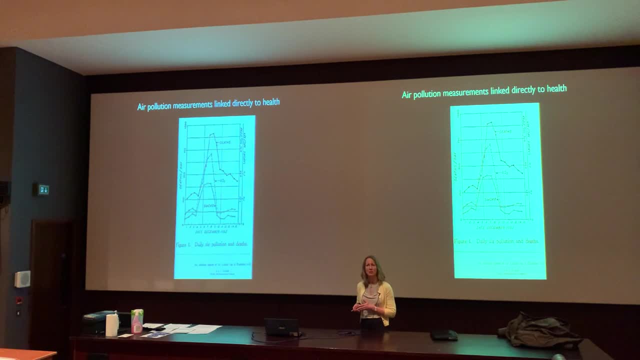 did start to develop some basic capability to measure some air pollutants, mainly through things like acid titration, So very basic techniques where they were able to start measuring gases like SO2,, NO2, and ozone. And this is the first academic record that 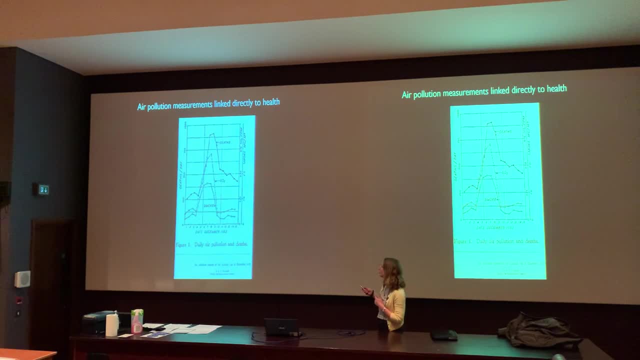 we have of the links. As long as you start being able to measure these pollutants, you can then start linking them to health. And this was probably well still to this day, the worst event in UK history for air pollution, which was the 6th of December 1952, where 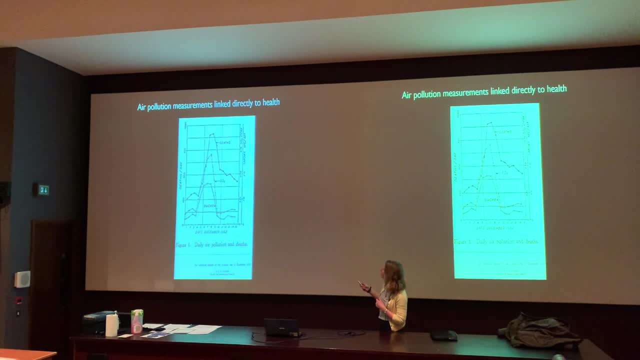 you see here the levels of SO2 that were measured alongside smoke and alongside the number of deaths per day that occurred during this absolutely awful episode of only a few days, where the atmospheric boundary layer, the atmospheric boundary layer and the atmospheric boundary layer, which basically means the layer which air is circulating around, was. 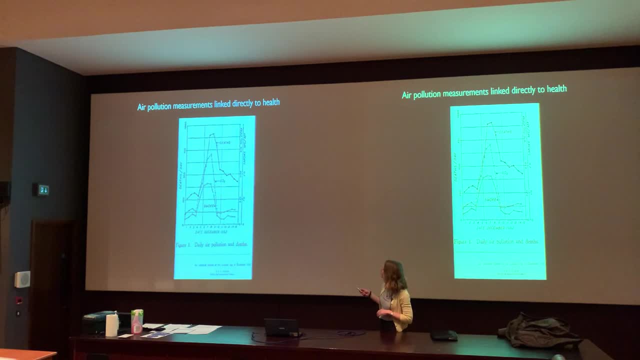 very low. so those pollutants were trapped and concentrated And we can see this direct correlation between these things happening. This is very rare to be. normally, in air pollution terms, you see a chronic illness developing over time with exposure to air pollution. But this was so bad that literally people were dying by the day, And the estimates here were up to 1,000 deaths per day. This is just in London And as bad as that seems. actually, the more recent estimates said the deaths were more like 10,000 per day, because these were only those people that got themselves to hospital. Most people did not get themselves to hospital, So that 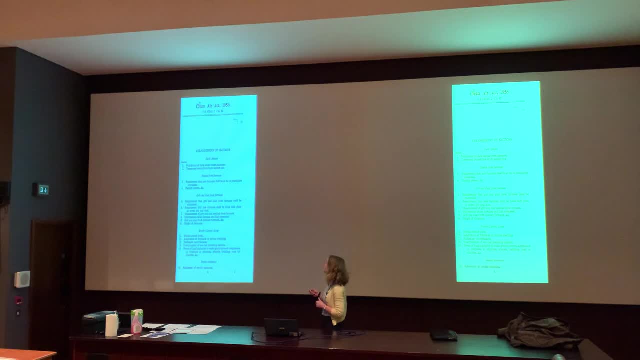 was absolutely terrible, But I suppose the silver lining is it was so bad that it did lead to the UK Clean Air Act. that happened in 1956. And this was the first legal instrument for putting in place- yeah, a legal instrument for putting in place, a legal instrument for. 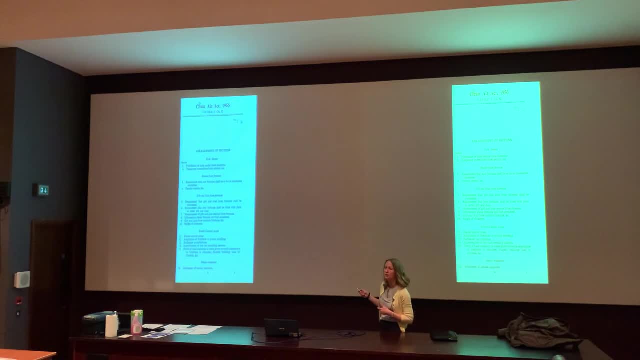 the legal act of reality for air pollution, all sorts of things that you then could not do. You couldn't just put smoke in furnaces in cities anymore, And this UK act led also to the US- the US EPA Clean Air Act as well. So they began to clean up their act for air. 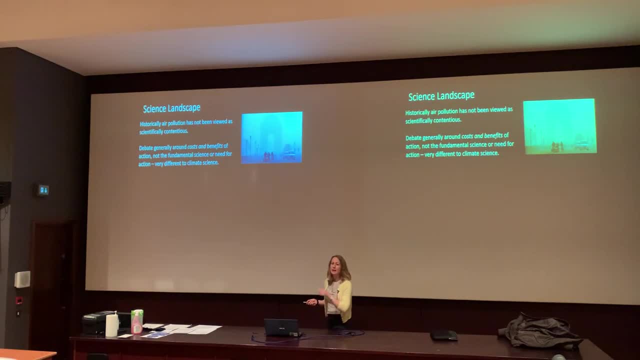 pollution a little bit later. Interestingly, it's worth thinking about where we are now. So I think what I've shown you is that air pollution has been around for a long time. It's not been really considered to be scientific. We may have debated around exactly how we should control air pollution or how much. 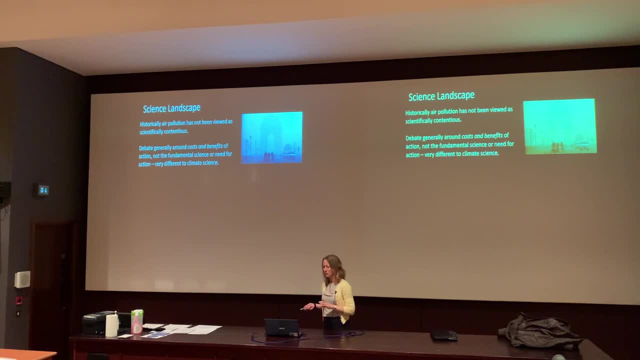 money we should spend or where we should put different things and how we should do it, But the fundamental science is not the question or the need for action, And that's very different to climate science, which has been very political over a long period of. 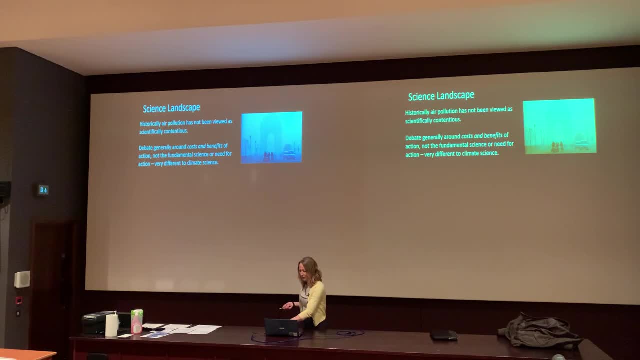 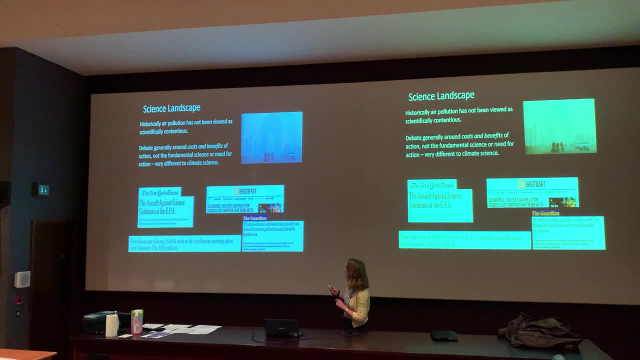 time. perhaps slightly less so now, But actually a few years ago it was rather different. We started to see this air pollution science being under attack. There was an issue- this is really from the old right, so an issue, an article in the Right Act, basically. 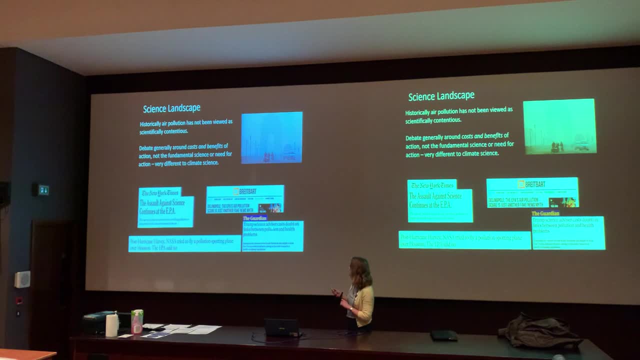 calling air pollution fake news and the Trust's Science Advisor casting doubt on the links between air pollution and health as well. And so you sort of think: well, why are they doing this? Well, clearly, the administration at that point wanted to carry on burning coal. 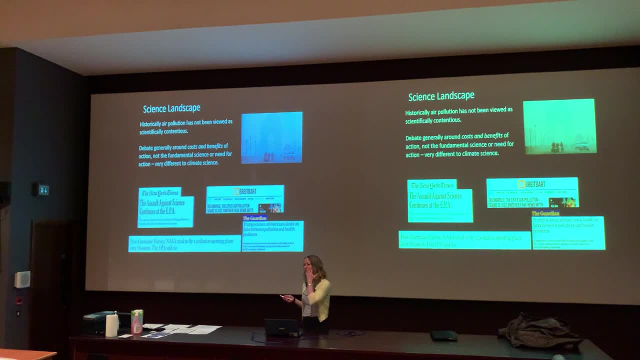 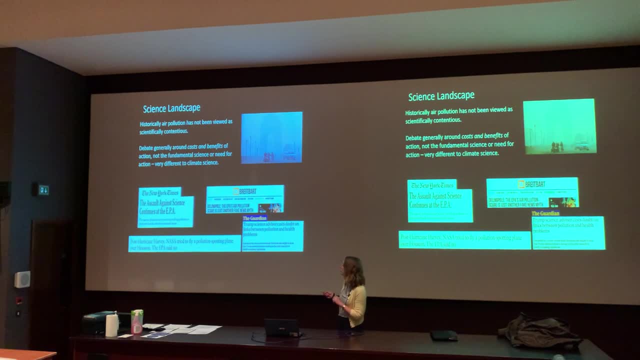 So if you want to start opening up coal power stations, coal-fired power stations, you have to attack the air pollution part of that policy, And luckily that never happened. Well, they were not successful in going through that case. They did not. 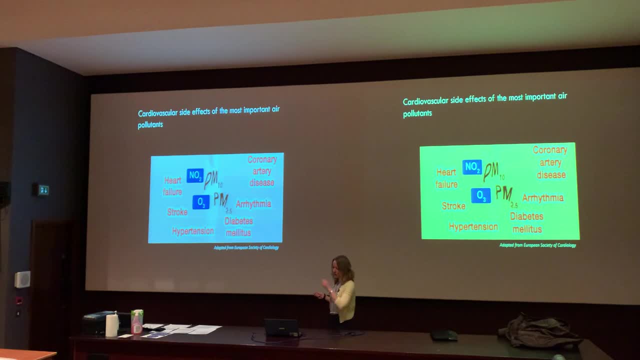 They did not, in the end, open them up. So these are. So what I would say is: the science of these links between air pollution and health are actually very well established. We know that the main air pollutants are. The most dangerous one is particulate matter. We often 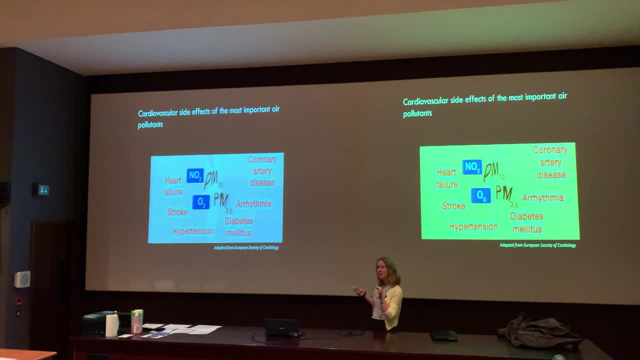 call that just PM. And PM10 is the larger particulate matter, particles that have diameters of up to 10 microns, And PM2.5 has diameters of 2.5 microns. So these are the two major particles that can get really inside your lungs And this can be formed directly from. 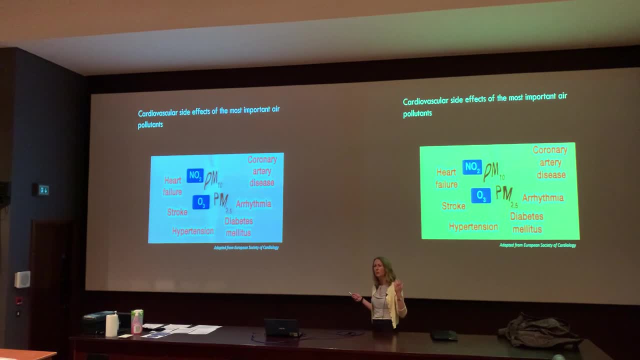 things like from combustion- from, say, diesel combustion or fossil fuel combustion- Or they can be formed in the atmosphere as well: NO2, another air pollutant, and that is ozone, which I've already mentioned- And the health effects aren't just limited to respiratory. 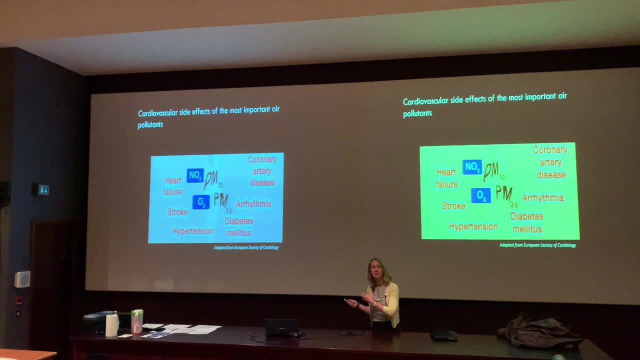 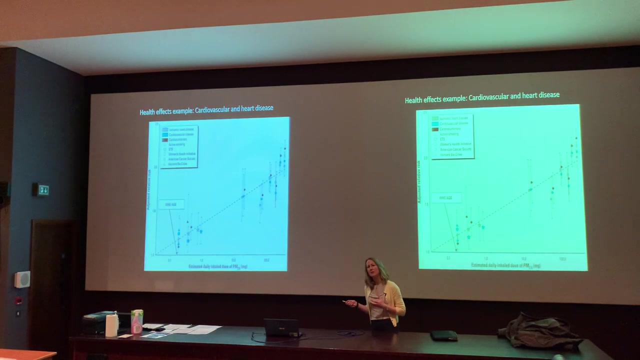 disease, Respiratory disease was a big thing. It was clearly even in the 1950 episodes- But things like heart failure, Hypertension, diabetes and also stroke. So there's a whole range of conditions that that can induce And the science now is sophisticated enough that we don't just know that there's. 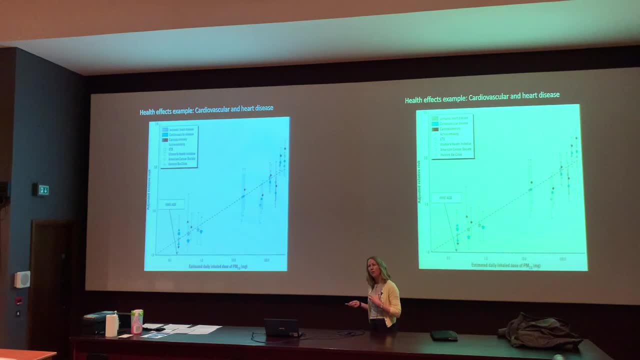 a link We can actually calculate the risk of someone contracting one of these diseases or the elevated risk of contracting one of those diseases for a certain increased amount of one of those air pollutants. And this is a graph which basically is used to make those sorts of. 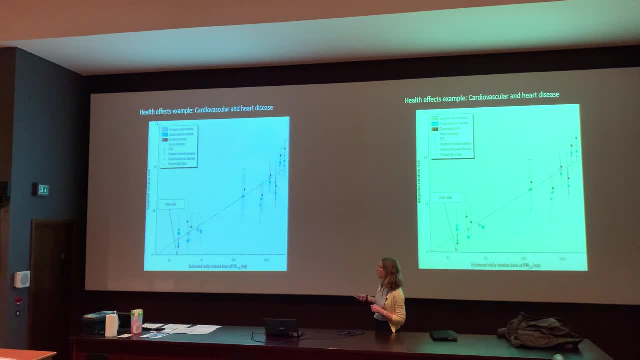 estimations. So we've got here a daily inhaled dose of PM2.5, so particles less than 2.5 microns in diameter. The data up here is actually- and this is your adjusted relative risk of contracting various of these diseases, different kind of vascular diseases, basically The. 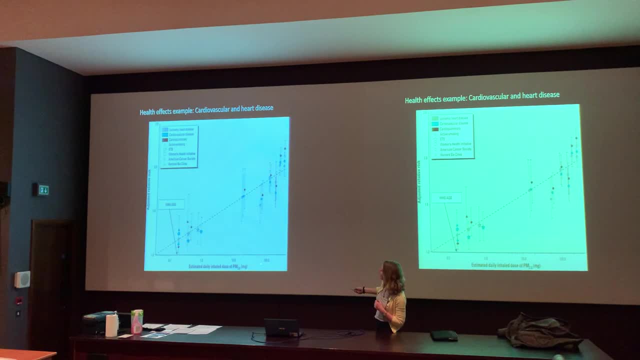 data up here is all from smokers, because essentially they're inhaling, you know, these daily doses. The data down here is from people living in cities, which in a way, is like having a small dose of smoking, And so these sorts of research. so this is data that's collected. 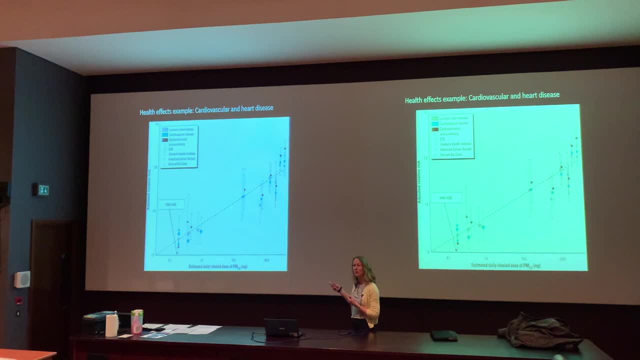 from you know, real epidemiological data correlated with the amount of PM that's used. So from these graphs then you can actually estimate how many people around the world are affected by air pollution And, as I'll show a little bit later, you can actually 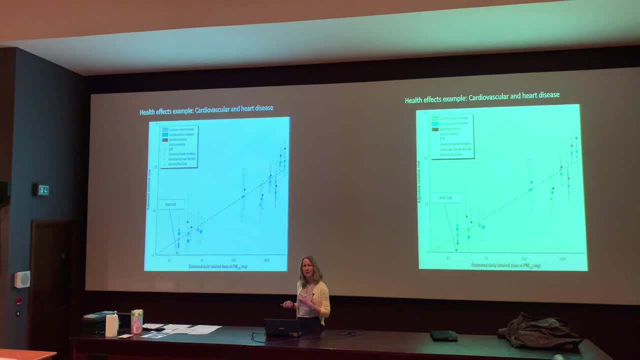 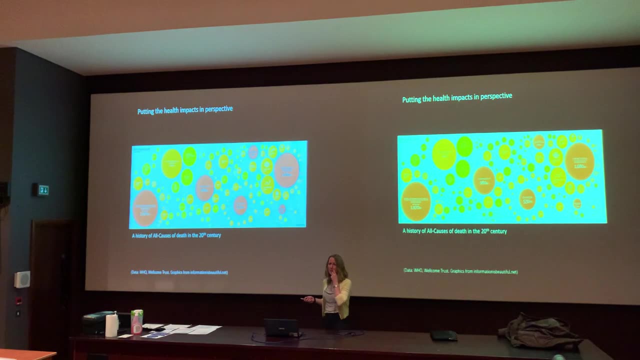 calculate the cost that it takes to treat these diseases, as well that air pollution causes. So just to put those half-impacts in perspective, this is a history of all causes of death in the 20th century. I know a lot of you do sort of medical biological specialisation, so you're. 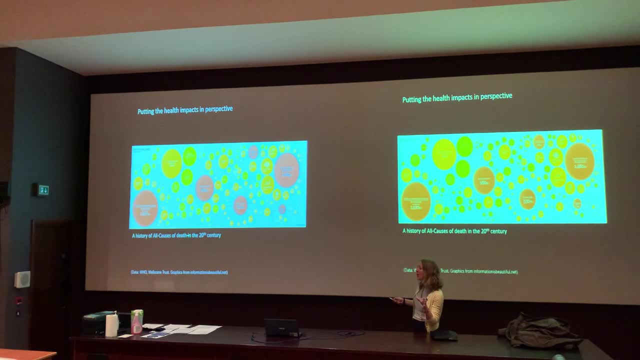 probably aware, This is not just in the 20th, this is integrated over the whole 20th century. so we may already be in a bit of a different place for the 21st century. But of course disease is the main killer, whether that's infectious or non-communicable disease. But death by humanity is about two-thirds of the total number of deaths in the 20th century. So death by humanity is about two-thirds of the total number of deaths in the 20th century. So death by humanity is about two-thirds of the total number of deaths in the 20th century. 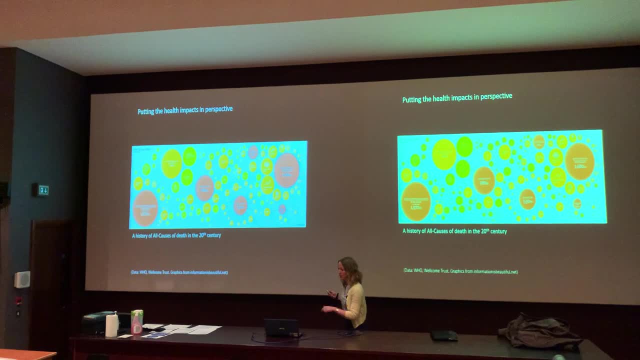 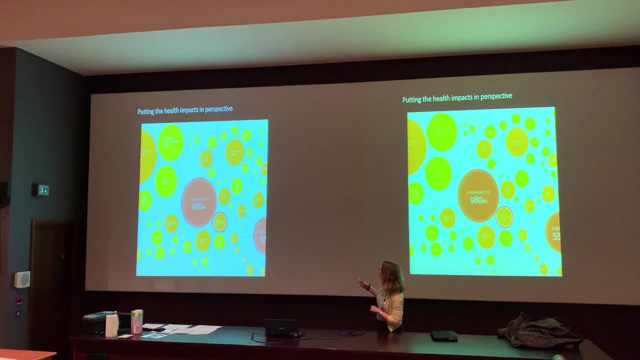 So death by humanity is about two-thirds of the total numbers of deaths in the 20th century. So it was about 20% of the total deaths that occurred in the 20th century. If we zoom in a little bit at what we mean by humanity, the main cause of that is accidents. 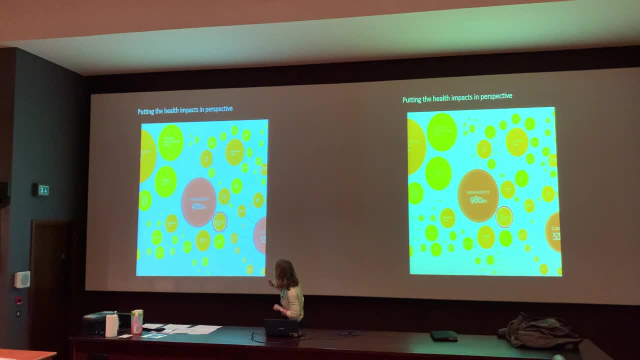 but interestingly, air pollution- I don't know if you can see that figure, but that's about 116 million- is very similar. Air pollution is the same number pretty much as drugs, as war, as murder or ideology, So it really does end up in the premature. death of a large fraction of the population, And that was, as I say, the 20th century. As we move now, we've got even more organisation and more people living in cities, so the fractional amount has got higher. even if it doesn't kill more people, in terms of numbers it will. in percentage terms. So the World Health Organisation, on a global basis, have calculated that air pollution is the single largest cause of preventable death by 2030.. I think it already is by now, And this is because 95% of people live in areas where pollution is above the. 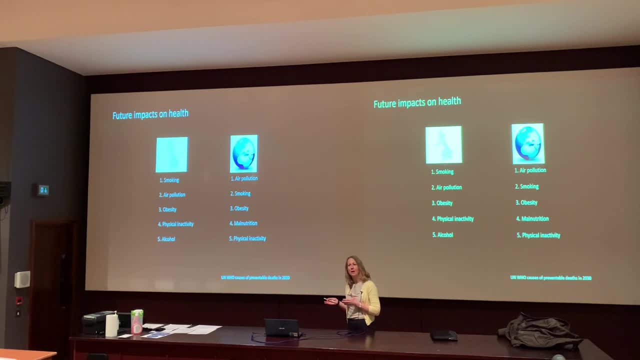 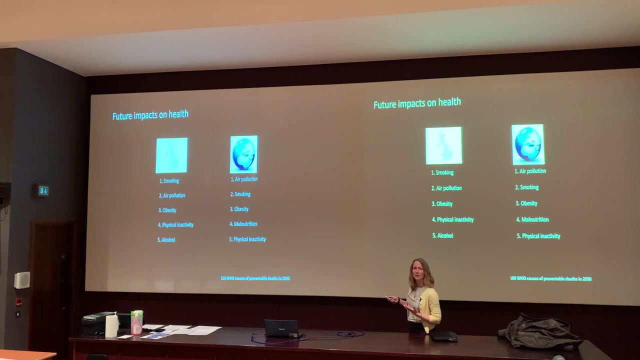 threshold set by the WHO, Not without the worst countries in Southeast Asia, I think. India has half of the world's top 50 polluted cities. China has eight, So that's way more dangerous for you than these other preventable deaths. In the UK smoking is still number one, even though I mean I don't know many people that. 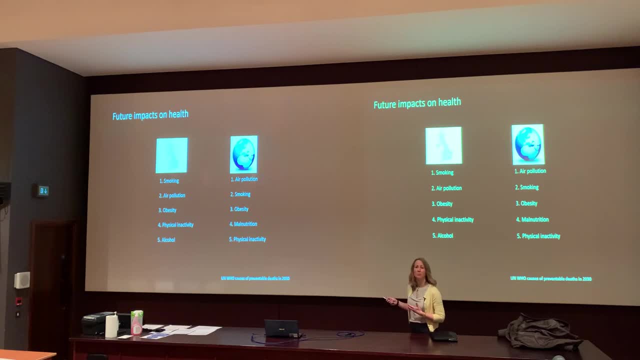 smoke. But you know air pollution is not such a big problem in the UK So it's not, so it's unlikely to be number one just because it's not. I mean, we're partly lucky because we live on an island so we have sort of cleaner air coming in but also have been regulated. 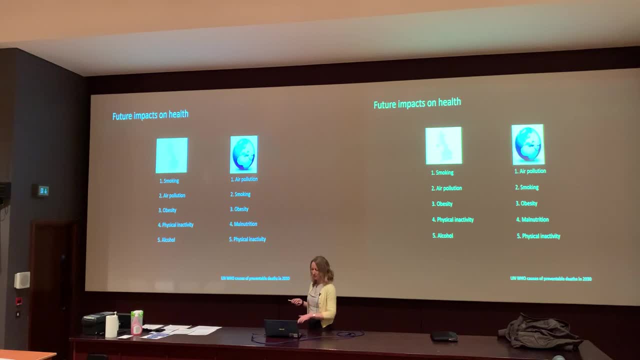 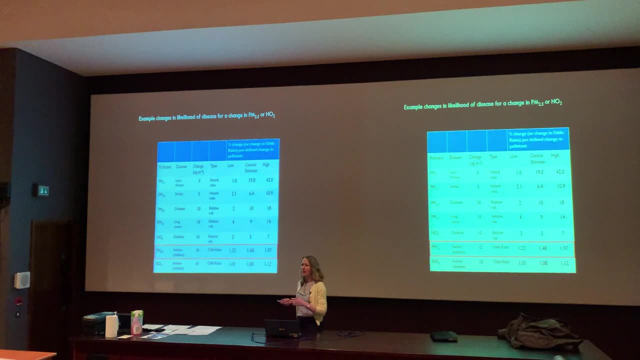 air pollution-wise for at least 70 years by now, And it becomes, I think, even more in the public eye. So, in terms of so, I think I persuaded you. hopefully you probably already knew that, yes, pollution is a problem that's worth solving If you're a government, if you work in government. 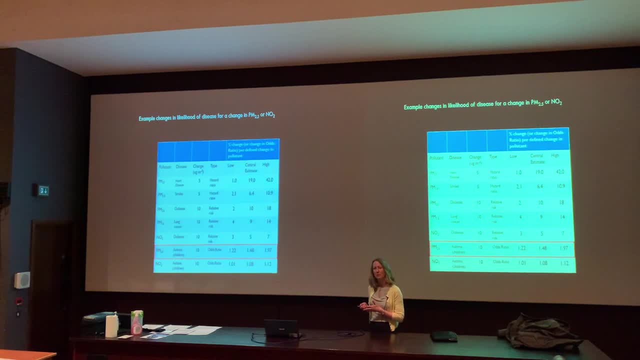 what you would ask yourself is: well, how much money should I spend to solve this problem? And then it comes down mostly to economics, as in most decisions, And so what you would do is you would do you basically work out what's the cost of air pollution to the UK. 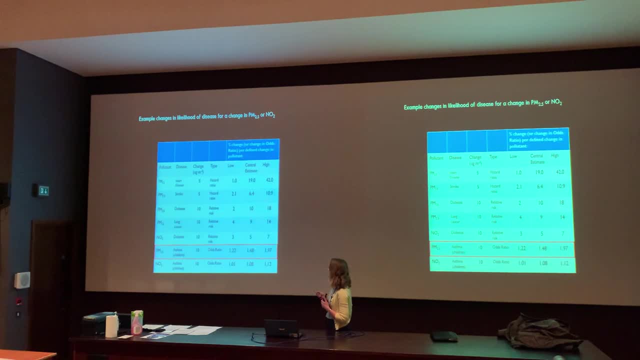 And from there you can use these data again. So, for example, if you look at the risk of air pollution, which basically gives you an increase or a change in risk according to a certain change in an air pollutant- So if we just take PM2.5, and we look at the change in risk of childhood asthma, So this 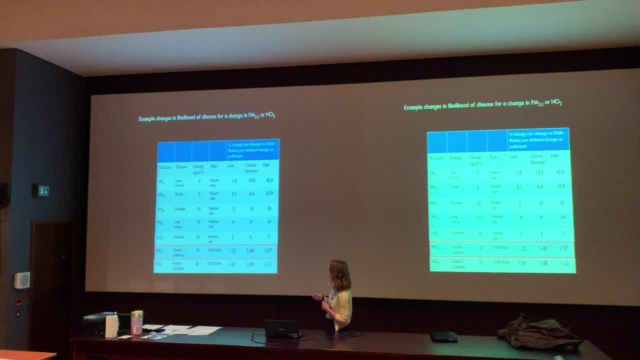 says that for an increase of 10 micrograms per meter cubed of PM2.5, the central estimate of that risk is it's gone up by 40%. Now we can actually calculate. now, of course, the health of the child is going to be a lot higher than the risk of air pollution. So 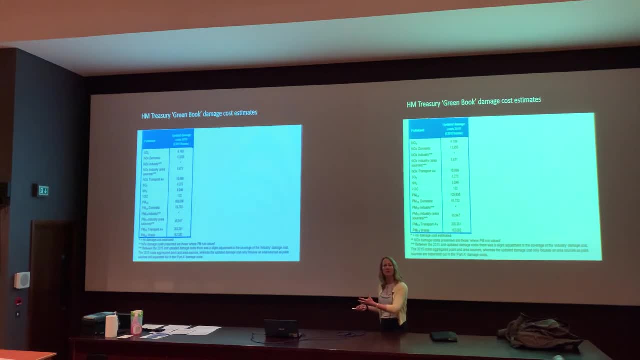 the child is unquestionably very worth protecting, but brutally they do put these numbers in value as well, so that they work out the cost. And actually from that you can. this is a socialization treasury, so-called green book, and you can work out because we know. the cost of treating asthma through hospital visits, through medication, et cetera, that every tonne of PM2.5 emitted by transport is going to cost 200,000 pounds And, interestingly, you can separate PM2.5 emitted from transport as a higher cost than. 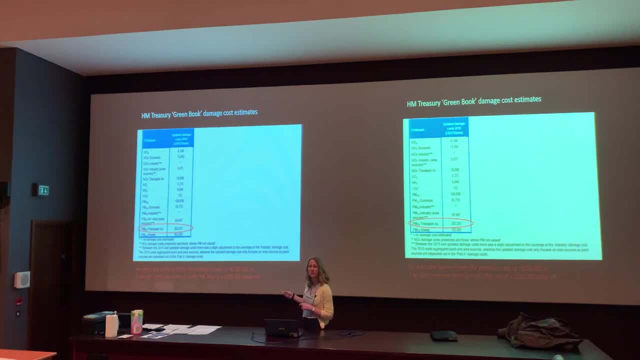 that emitted by industry, and that's because people are more exposed to the emissions from transport, obviously, and further away, in general, from industry. So that's how these calculations are made and you know the UK, amongst other countries, has been persuaded. 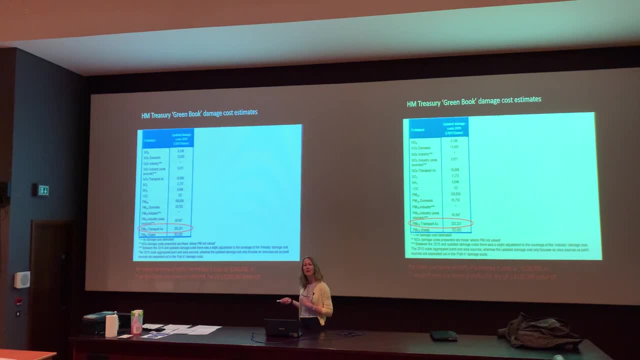 for a long time that it's a problem worth fixing and they have an idea of how much they want to spend on it. according to that, It's much more difficult. It's much more difficult actually, for climate change, where there are so many feedbacks that go on. It's harder. 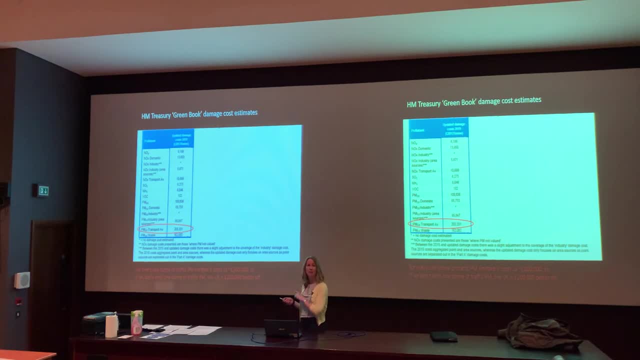 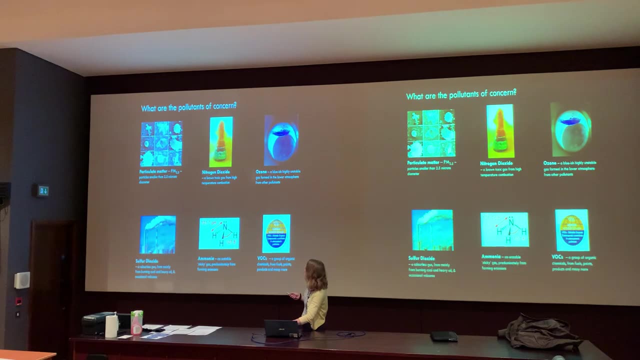 to calculate all of these risks to such certainty. Here you rely on medical data, which we have a very good idea of. The main pollutants of concern are these six. So I mentioned particulate matter, Na2, ozone, sulphur dioxide. I've mentioned a little bit from coal Ammonia. 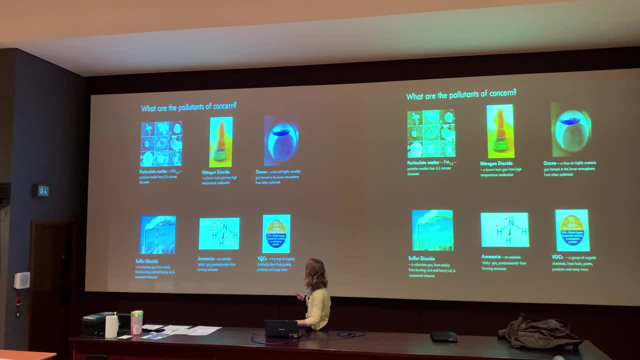 is also a pollutant. This is mainly from farming emissions. These are a catch-all term of volatile organic compounds. These are basically hydrocarbons from fuels and paints and other things. So these are the main six and it's a bit complicated. 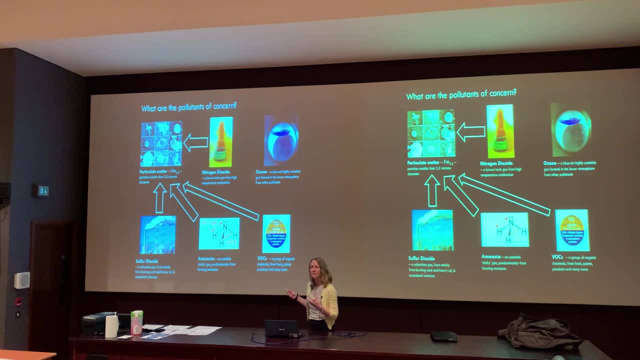 because particulate matter, as I said it, can be formed directly from combustion, but also all of these other atmospheric pollutants can form particulate matter as well. So there's a lot going on that, as chemists, we need to understand to try to predict what's going. 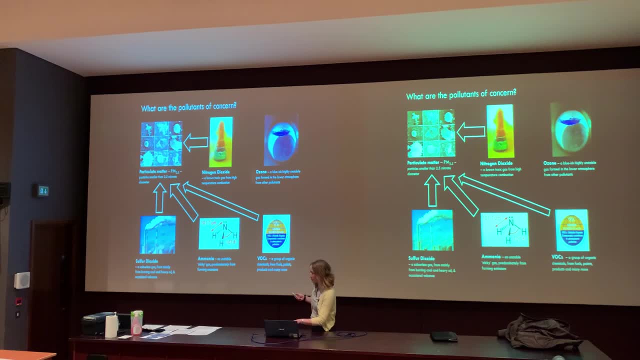 to go on in the future if you change any one of these emissions. And then ozone- and again I'm talking about ozone at the surface, where it's a pollutant is not emitted directly, but it's formed from nitrogen oxides and from these VOCs, so things. 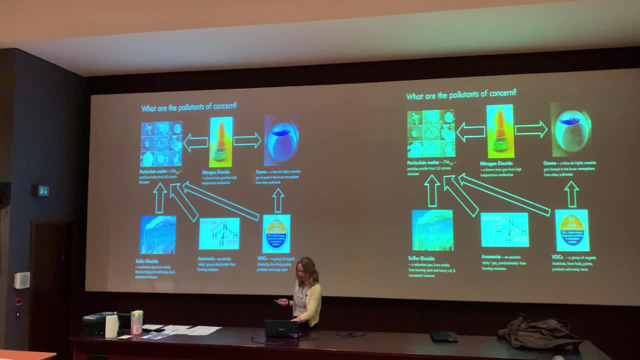 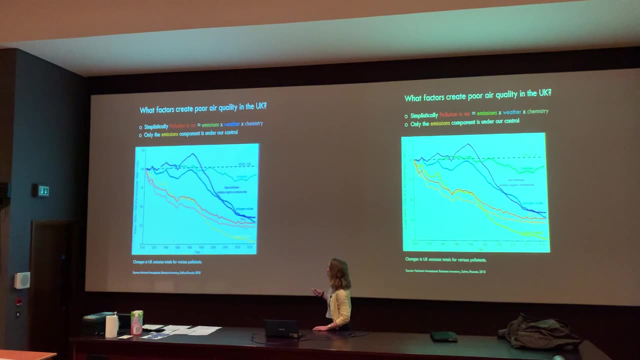 like ethane and propane and benzene, so they go on to form ozone, So they're the main pollutants. Now how have we done with those over time? Well, you can only really look at how we've done with emissions. So, in a simplistic way, the pollution that you experience, that you 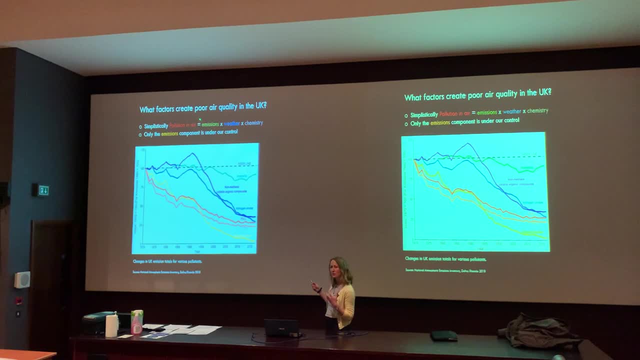 see in the air is basically a product of the emissions times, the weather times, the chemistry. Clearly we don't have much control over the weather. The emissions is a bit we can control And if you look back from the 1970s you can see that there's been a lot. 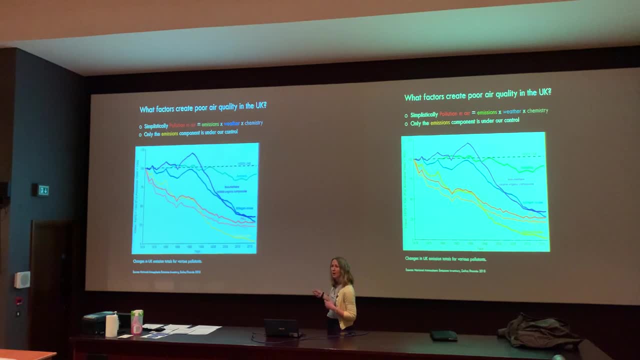 of success, particularly with sulfur dioxide, SO2.. As I said before, that was relatively easy to control because you can remove it from coal-fired power stations, and we've only got one or two coal-fired power stations left now anyway, so I think it's about one. 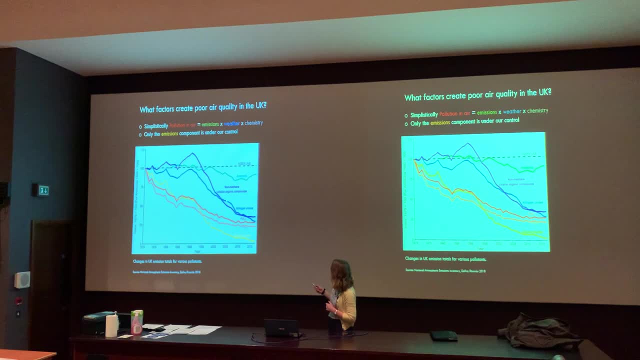 percent of our total energy use. Volatile organic compounds: the VOCs have also come down a lot, so that's pretty good. Ammonia isn't looking good. This is hard to regulate because it's sort of a product of putting fertilizer or using it in farming, so it's 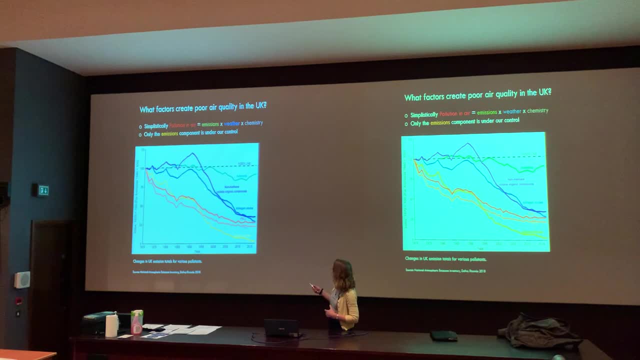 harder to regulate. Nitrogen oxides don't look too bad, but we're not doing as well as we should be doing, especially compared to other countries And the most dangerous pollutants, these PN and particulate matter, is really kind of just a little bit of a. 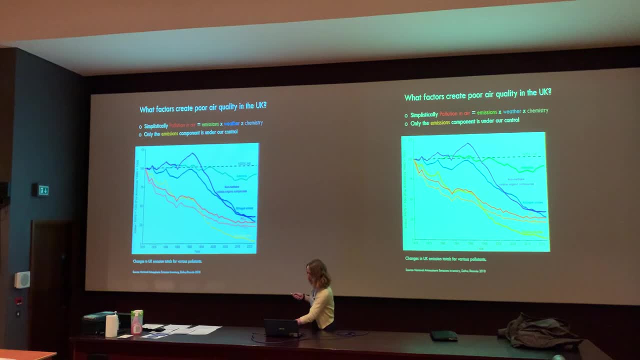 little bit of a problem. They're just flattened out and they're not really making as much progress there. In fact, the UN- I don't know if anyone remembers seeing this, but a couple of years ago- I think it was the pre-pandemic days- really called out the UK. 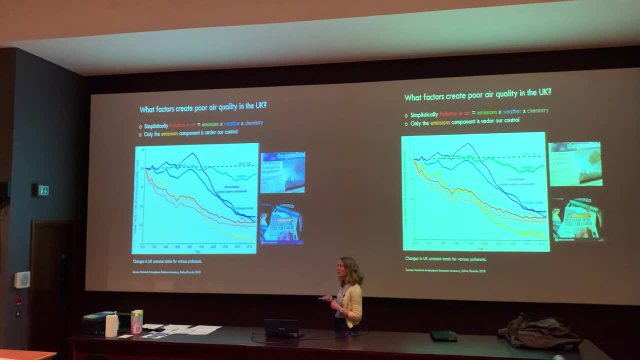 and said: you're doing really badly on pollution, particularly in disadvantaged areas. So it's an issue that does discriminate more against people living in poverty. So yeah, so we're doing okay, but we're not doing brilliantly and there are still large problems, particularly 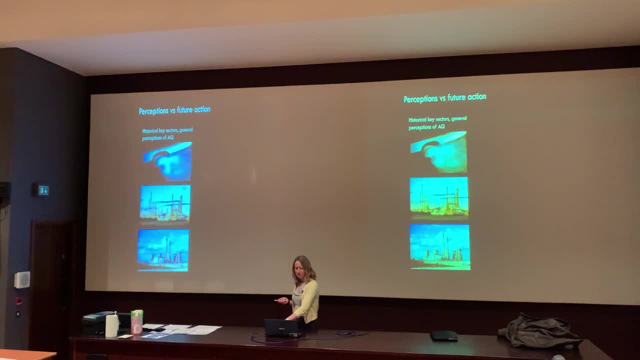 in cities with NO2.. If I was to ask you what you think about your main emission sources, I'm just going to guess that you probably think about things like your cars, your passenger cars, industry and, again, coal-fired power stations. Actually, none of those three things. 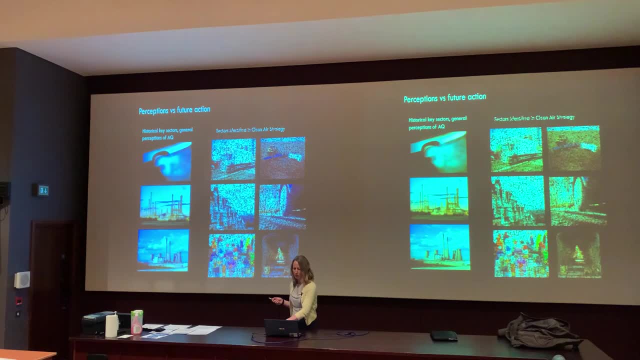 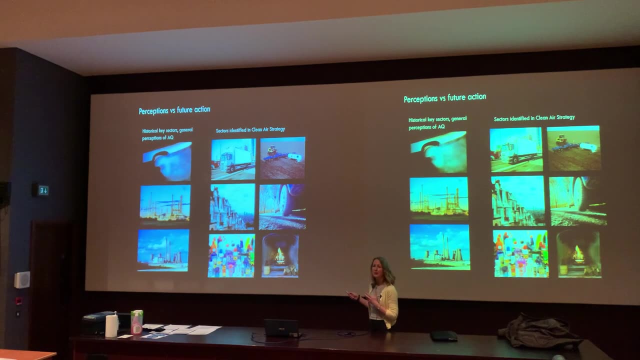 are in the UK policy going forward in the clean air strategy for the future. The reason for that is We believe that, you know, in the next 10 to 20 years the passenger car fleet will be electrified. We shouldn't have these same emissions. Industry has cleaned up a lot. 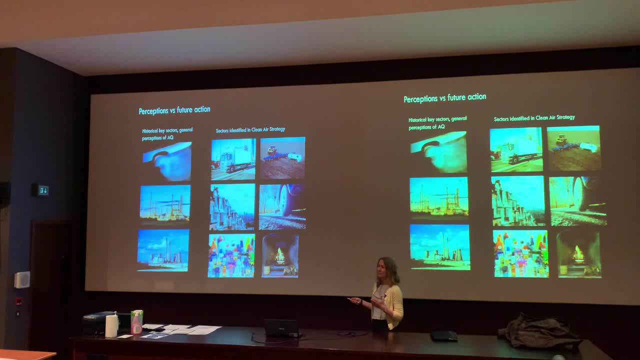 and, of course, as I said before, we've almost- you know there's very little Certainly now. who knows whether that decision will be reversed. we'll see what's going on at the moment, but we're down to, you know, a real rumbling of coal being burnt within the 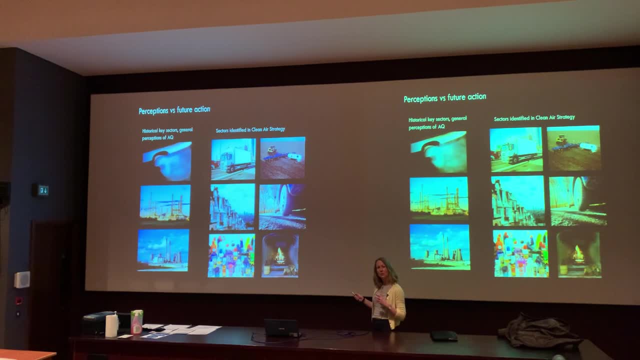 UK. But these are the sectors that now we have to concentrate on. They're quite different to the ones we've had in the past. We've got heavy vehicles that still often allow Transport vehicles- allow to, you know, rumble through cities. We've got farming, big production of ammonia. We have domestic 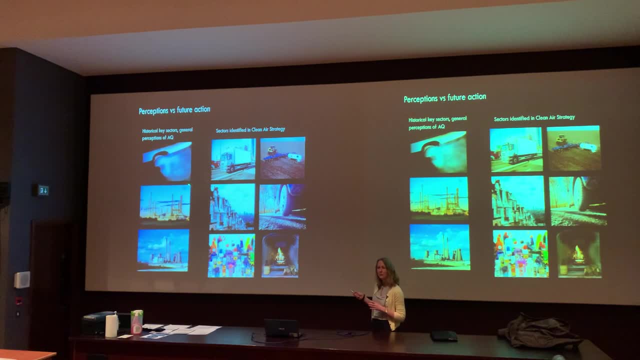 heating. We're pretty bad in the UK. We're really bad for insulating our homes. We need to get better at that. We've got brake and tyre wear, So even if you have an electric vehicle, the particles can be generated by the action of the tyre on the road. so that's. 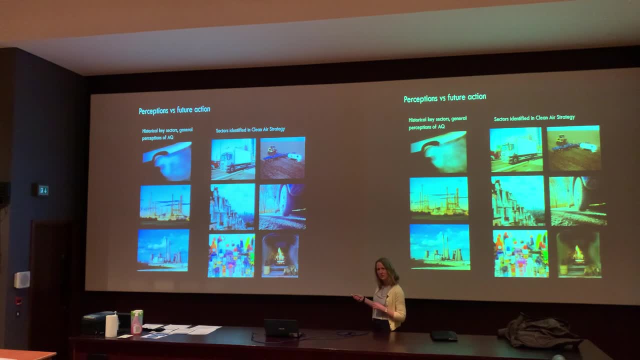 still an issue. We've got solvents and consumer products- a whole bunch of stuff here. We've got industrial and consumer products, BMCs, and we've got wood fires, sometimes called the Notting Hill effect, where everyone's got their own wood-burning stove. So it's kind. 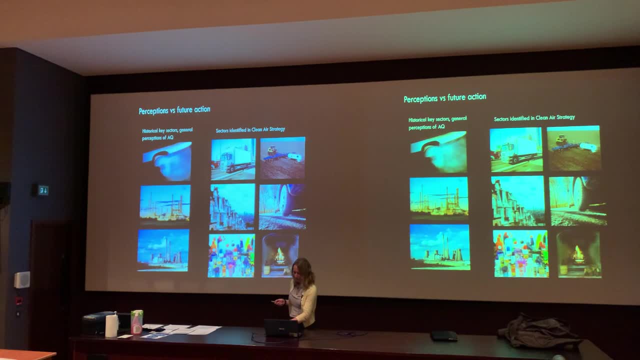 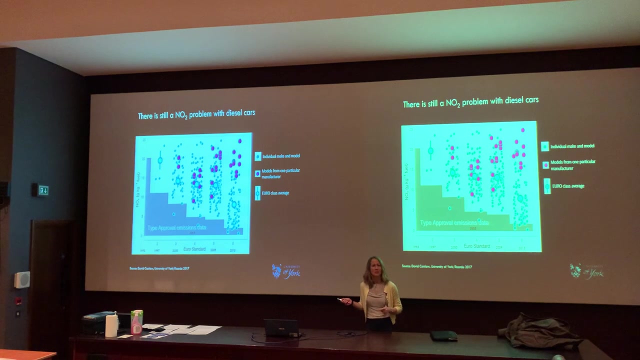 of a more localised pollution issue, But they are the main thing. So I'm just going to say a little bit about the car issue- diesel- and a little bit about VOCs as well. This graph comes from someone who works in York, an academic called David Castle, who I think has done. 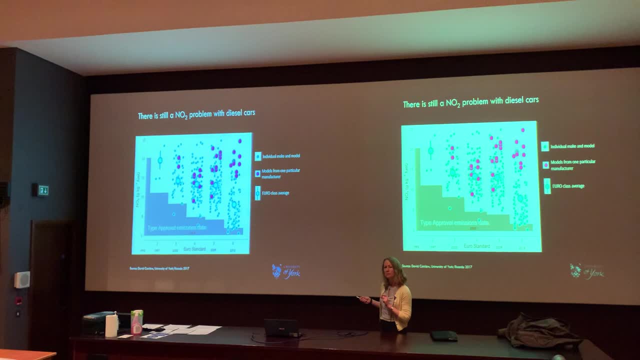 more than anyone else. He's done a lot of work on the car issue. He's done a lot of work to expose this dieselgate scandal and what it's meaning for NO2 emissions. This is from his data, So what we've got here is the NOx emitted by each car, and this is really 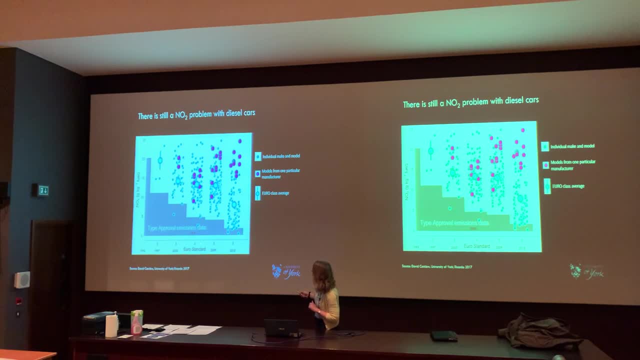 the function of year by Euro standard. So in other words, if you're, I don't know quite what's happening, I can see it on mine. but if you were driving a car, let's say, that was built in 2000,, you'll be on Euro 3 standard and these grey masks here show you the amount. of NOx- nitrogen oxides- that should be emitted by that car. So if you were driving a car according to the standard, clearly those emission controls are almost stringent. there's a years of on-pass and the Euro 6 car should be a lot better in terms of its NOx emissions. 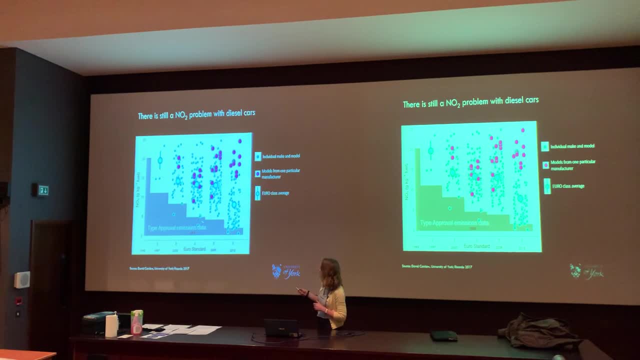 than the Euro 3 car. So that's the theory. that's what it should do. that's generally what they do in their IoT, but you probably guessed it, this blue data is what they actually do on the road. So David has basically detected by LiDAR the NO2 emitted on roads and you 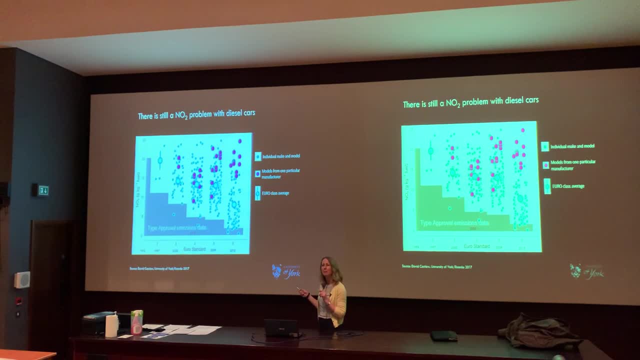 can actually detect through cameras So you can tell what the model is, you can tell what Euro standard it's under and these blue circles here are the average Euro class average of all measured cars over these different Euro standards and you can see that they're all way above what they should be and that 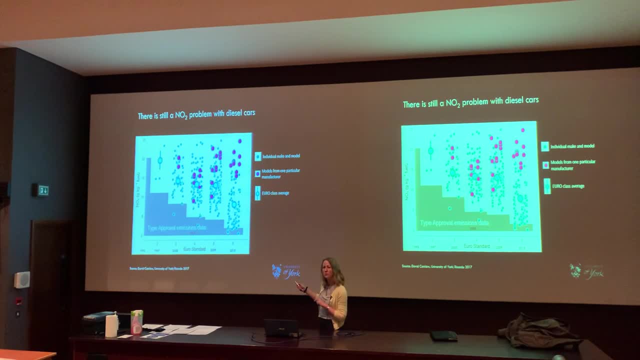 for at least 10 years, there was no progress made at all on the road, whereas the Euro standards were coming down, And so you can see there's a general decrease. but this pink one here are the models from one particular manufacturer. It's actually getting worse with time and it's not VW. So, thanks to David, these people 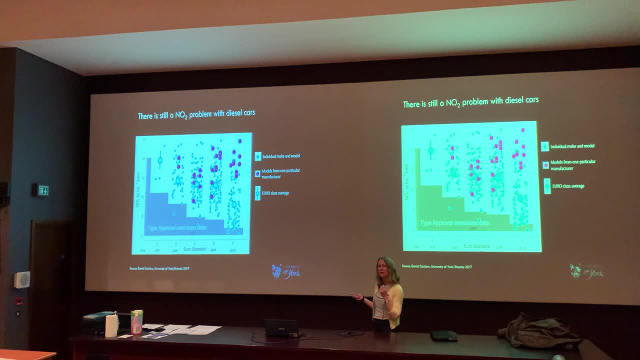 have been hunted down and the correlation between the cars that are emitted on the road and how much NOx they're doing is tightening up, but there is still a big problem with NO2 with diesel cars. It is getting better because the scientists have found ways to. 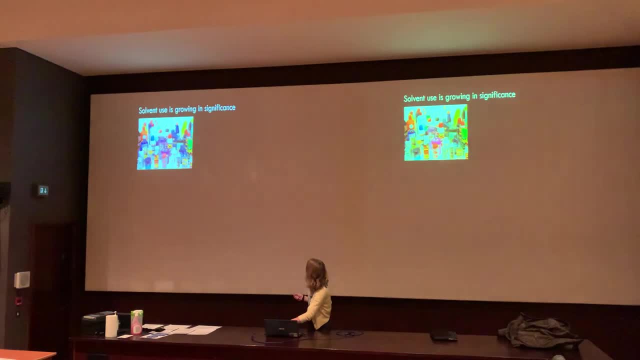 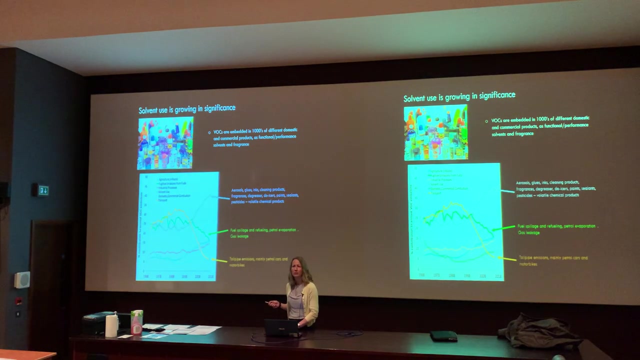 actually pinpoint what's going on in our cities. And the other thing I wanted to point out is around solar venues. There are all sorts of products that you will have in your own home. I don't know whether anyone here uses deodorant, for example, So no one in Cambridge uses deodorant, but if 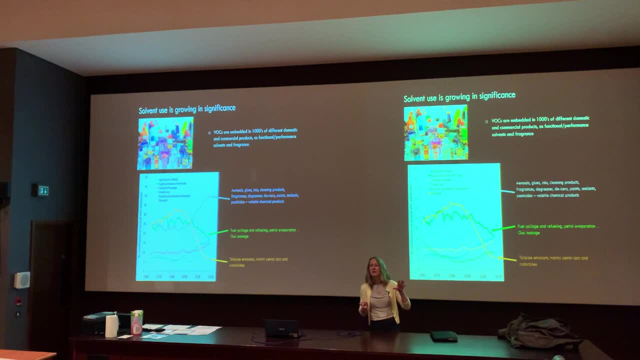 you do and if you use a spray deodorant. so back in the 70s if you used a spray deodorant it would have had CFCs that are found for good reason If you look on your can of spray. 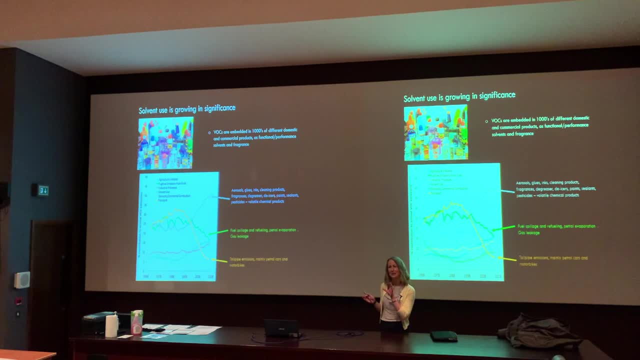 deodorant. maybe you're- hopefully you don't. maybe you use a stick. that's good stick with a stick, But you've got butane in them And actually if you were to drive a small Euro 6 car for about 15,000 kilometres a diesel car. your emissions from that car are probably quite similar to one can of deodorant spray of butane. So hopefully that persuades you, if you are using the sprays, to use the deodorant. Oh, not at all, that would be up to you. But the 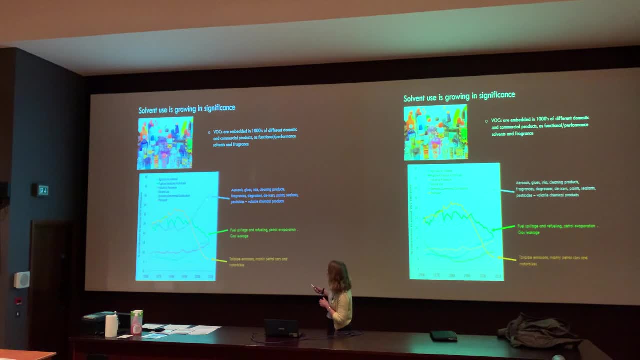 point is is that these, this sector, which we used to really not worry about, is now very efficient at getting rid of the VOCs. So the VOCs that are emitted from glues, aerosols, personal fragrance products, cleaning products have really come up whilst we've controlled. 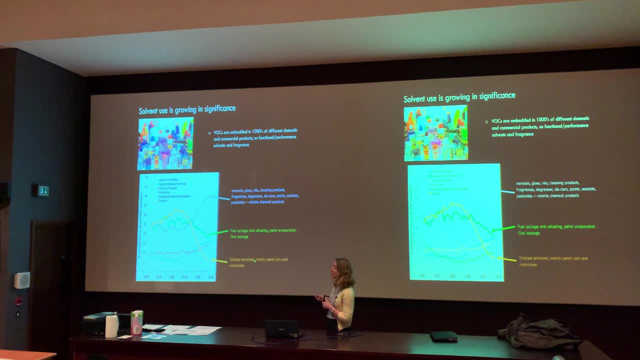 a lot better these VOCs that have come from the back of cars, And that's mainly. but the success there is mainly due to the use of a catalytic converter, which is now very efficient at getting rid of the VOCs. But this is a sector that really is kind of just just rolling. 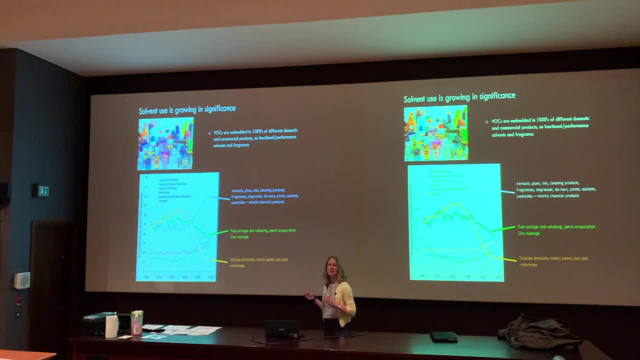 round and round without really people realising. So I think, in terms of what you can do in your own home is well, I always say: don't keep your home so much. Don't you actually do the environment a favour there? Finally then, I mean it's not finally, so we haven't got on to the last little bit, but in terms, 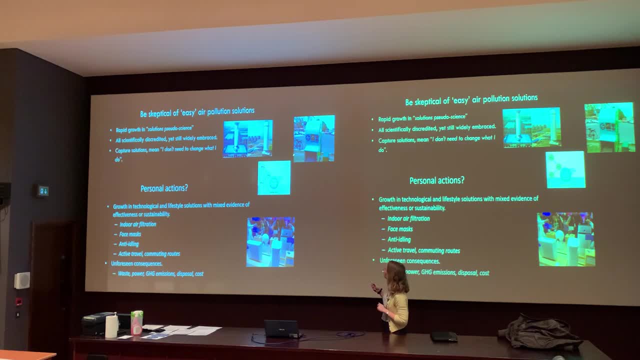 of this part of the talk. in the last few years there's been quite a lot of talk about these different solutions to air pollution. So things from NOx-eating to taming paint, to roadside air filters, to smoke towers- these precise solutions to air pollution. All of them might have a little bit of truth in them, but none of them are really going to get rid of air pollution efficiently enough. Partly that's due to the fact that if you emit a molecule of NO2 in the ground from a car, it typically mixes up to about a kilometre. 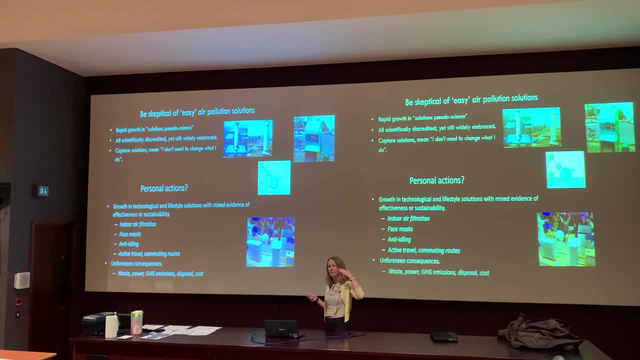 in the atmosphere. You can't stop it doing that. that's just atmospheric mixing. So if you've just got a point, source or a small place where you're trying to destroy that molecule, it really is just so inefficient It's not going to do any good and it's a sticking plaster over the problem. And then 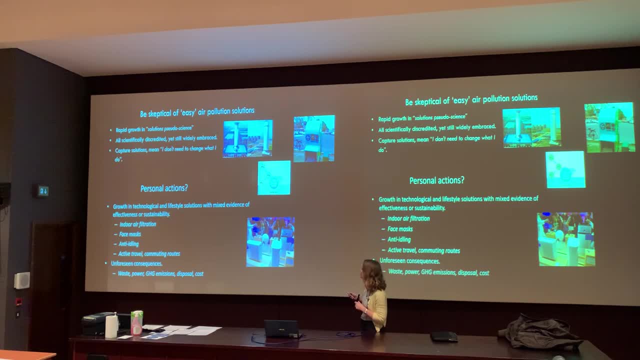 people. there are now personal actions, so indoor air filtration, for example. That may be quite effective at reducing the pollution in your home, but of course there's an energy cost. You're also causing now CO2 emissions somewhere down the line without electricity. 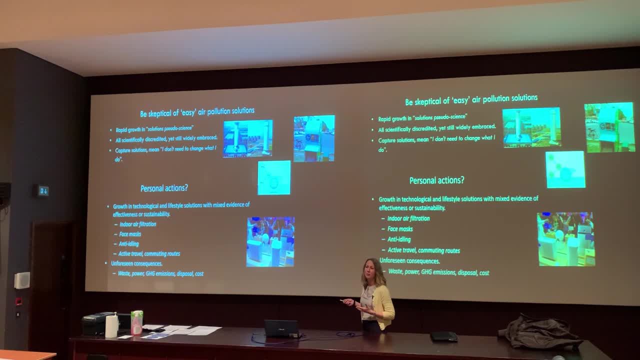 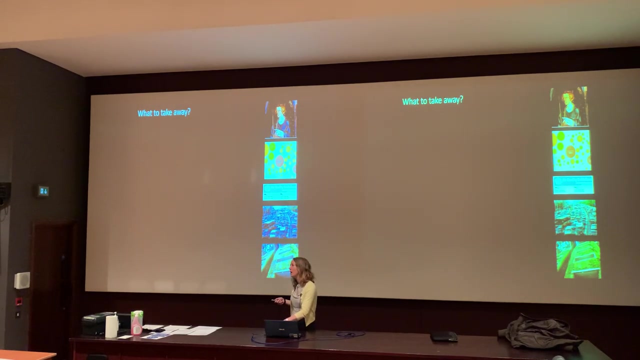 being generated. So, of course, really the problem has to be fixed at source. We need to stop emitting this many air pollutants rather than try to capture them once they're already in the atmosphere. So I'm just going to summarise this part of the talk, but before we go on to the bit, 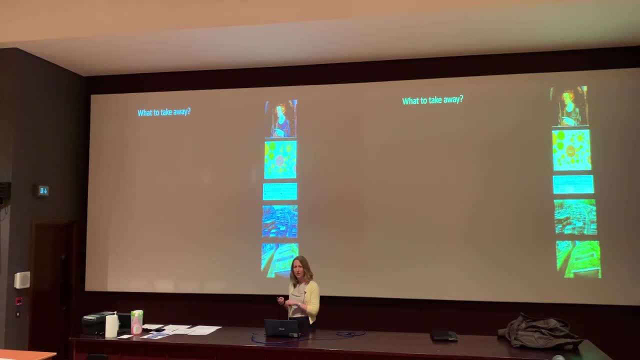 which is really the clean atmosphere, the remote atmosphere, which is where my research specialty is. So I've said lots to take away from that bit. Well, air pollution's been around for a long time. The health costs are real And the economic cost even in the UK and we've tackled it pretty well, is still around 6 to 11 billion a year. It costs us a lot of money. The passenger car problem is likely to resolve itself in the next one to two decades And again, if you see your local council- I don't know- proposing these sorts of issues, beware. 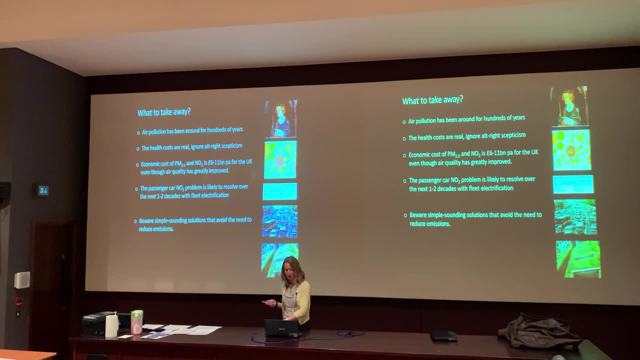 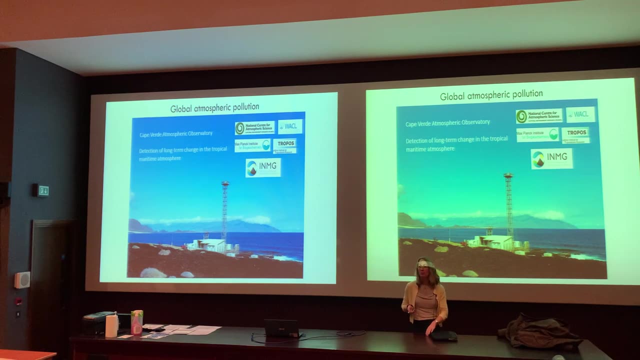 because they're probably best than they actually are, But they sound best than they are. Okay, so that was really about the pollution that we see in cities, where most of us spend most of our time, And we ought to be aware that the health costs are real, And I think 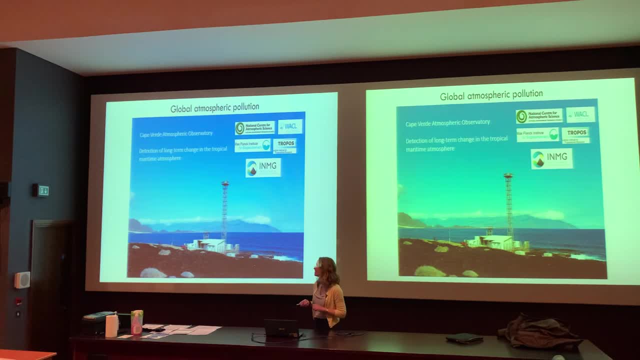 the health effects are real and even in the UK there is an issue, but we are lucky compared to some countries. But I spent a lot of my research career looking at what's going on in really remote places And actually, if you're trying to monitor the long-term compositional change of the 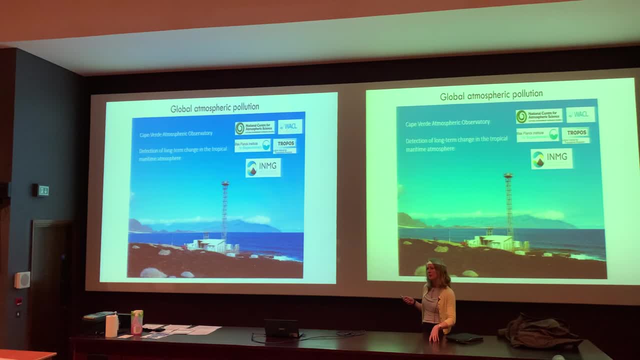 atmosphere. you can't just be monitoring sitting in a place next to a pollution source, because you'll be dominated by that one pollution source And if you want to measure long-term changes, you want to be in a place that sort of is a long way away from that pollution. 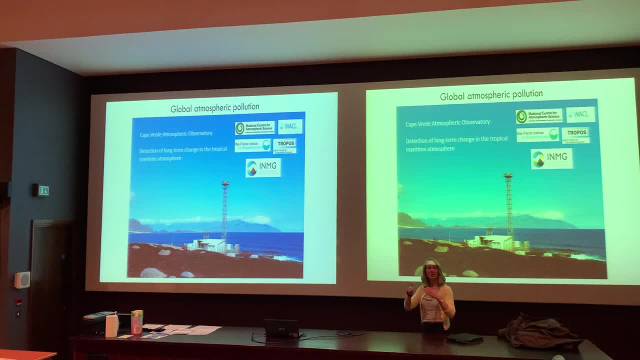 where it's all integrated and mixed up together and you can measure a representative part of the atmosphere where any long-term changes are due to a whole global scale or hemispheric scale changes. And that's what we've done. We set up an atmospheric observatory in the 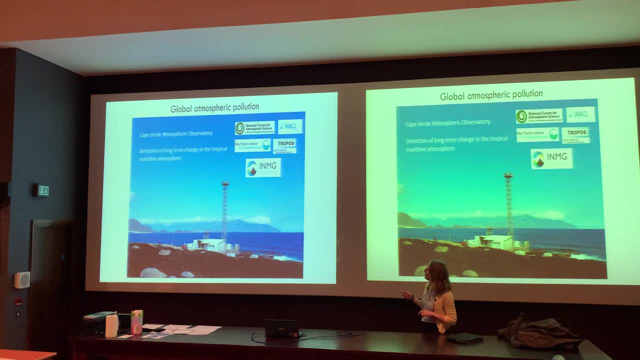 Cape Verde Islands. I'll show you where those are in a moment, in around 2006.. And I'll show you some of the things we did discover. So this is what we're discovering from this observatory, which is a collaboration between: 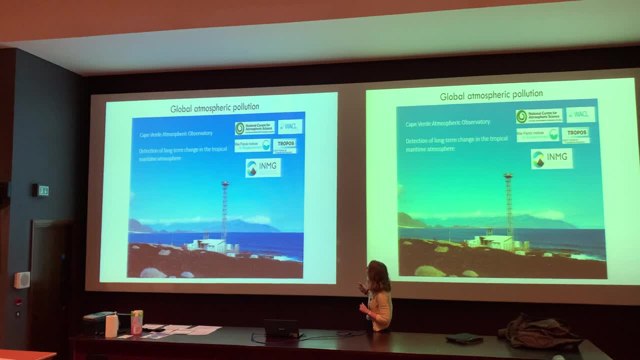 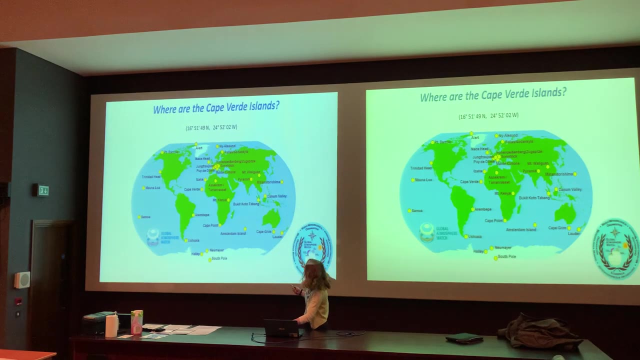 us at York, two German institutes, the Matplank Institute in Nona and the Tropos Institute in Leipzig, and our Cape Verde partners on the island of San Vicente in Cape Verde. These are basically the next office of Cape Verde. Here it is, And it shows Cape Verde on a map. 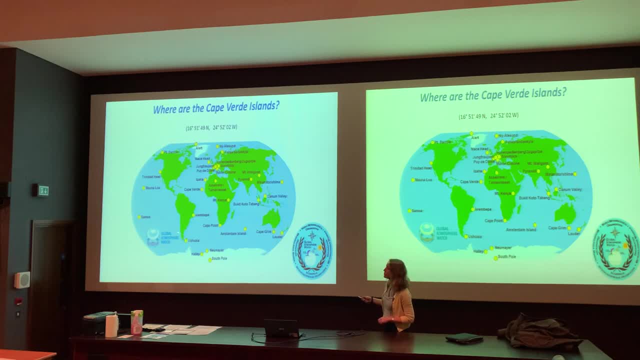 of other so-called global atmospheric watch stations Which are this sort of UN global atmospheric watch stations. There are around 30 of them around the world And you have to have a certain quality of your measurements and you have to put them into a database and you have to do that yearly and there are 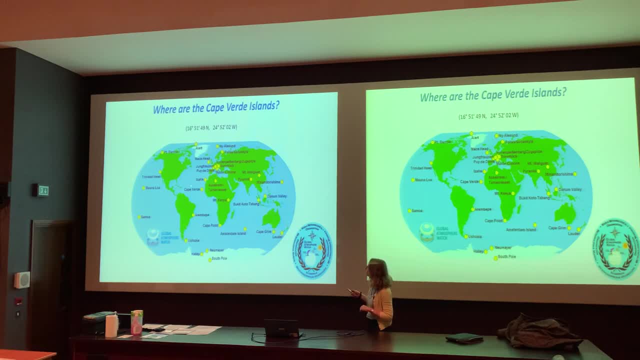 all sorts of these requirements to do that. But that's where one of those- and there aren't many in the tropics and the tropics is particularly important because that's where a lot of chemistry goes on to kind of get rid of some of the pollutants that we see. 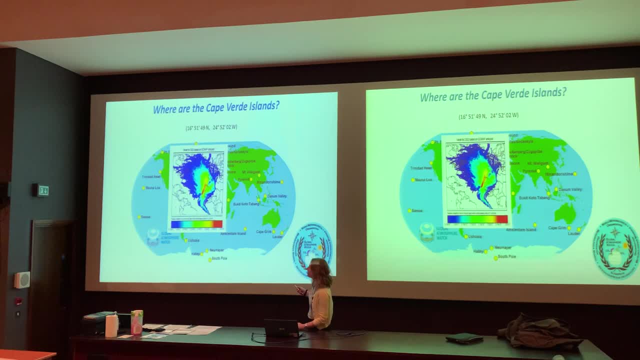 This is a so-called back trajectory map that atmospheric scientists love. So that little black cross, there is the position of Cape Verde, And this is a sort of footprint of the air that arrives at Cape Verde. So the warmer they come up, the more frequently the 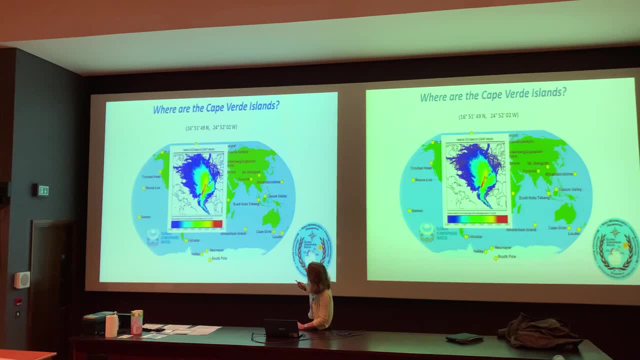 air arrives in from that direction. So nearly all of the air comes in from this direction. it comes from the northeast. That's because the air is mixed around the trade winds and comes to us from that direction. But you can see it picks up along the way. this is, I think. 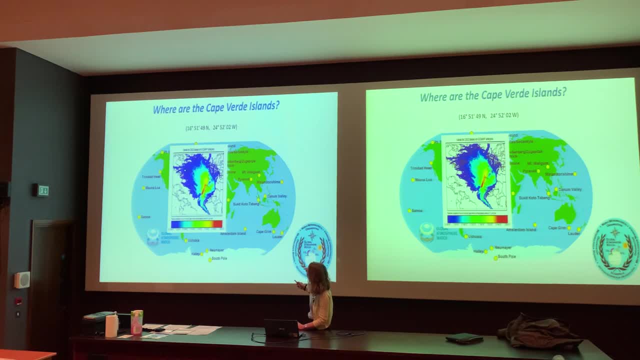 a five-day back trajectory map, So where it might have been five days before It picks up air from North America, from Europe and from Africa. We see a lot of Sahara dust at certain times of the year. Occasionally we get air from the southern hemispheres as well, So we did it sort of monitoring those. 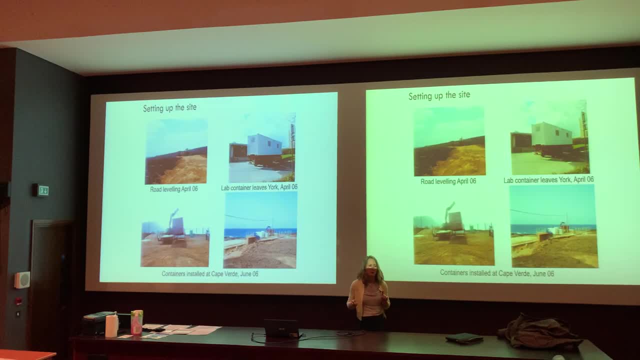 kind of background levels, And we're very proud of this observatory, not only because it's a great place and we've discovered some good things to measure these compositional changes, but we really set it up from scratch on a piece of lava rock, So there was nothing. 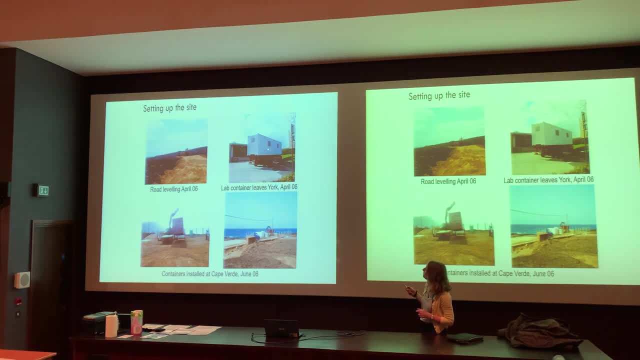 there We had to build a road. All of the labs were basically equipped from converted shipping containers at York, put on a ship, sent to the site. You can see this rock that we've got here. You don't want to go over that bare feet. I can tell you We were right by the 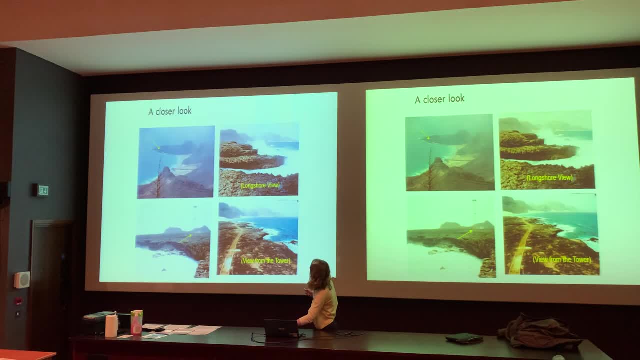 sea. We had to park power lines as well. That's where we are. I mean, it's a beautiful site, but the observatory is there looking out right into those trade winds, So we get air from the ocean all the time, which is fantastic. 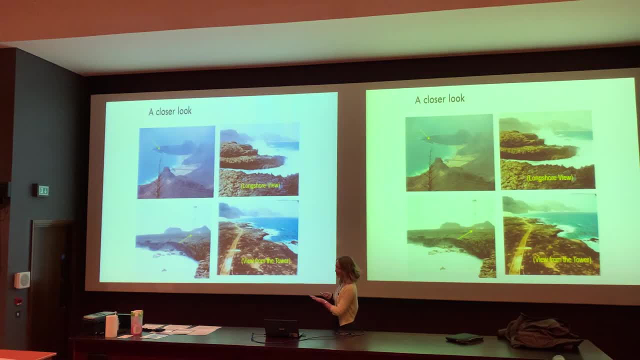 I'm always trying to tell if it's going to be in there, And that's the road that we've got to take. It's an island that has a wet season lasting about two weeks a year, So in September you might get some rain. the rest of the time, if it doesn't rain, This is what. 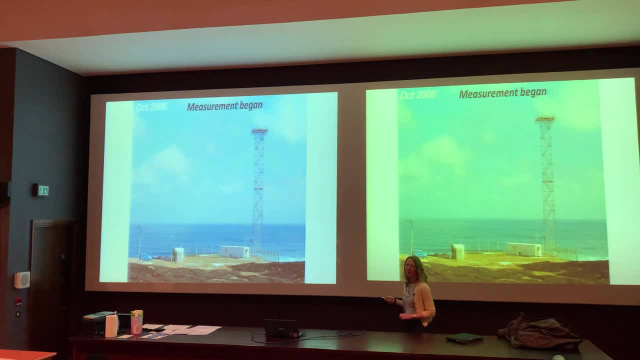 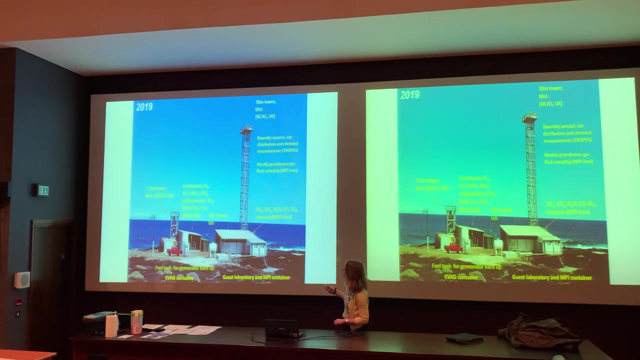 it looked like when we first set it up. It looks a little bit like a sort of graveyard for shipping containers with a big tower. It looks a bit more sophisticated now. So this is the UK part which we measure all of these different things continuously. So ozone, VOCs, NOx, hydrocarbons, SO2, CO2,. 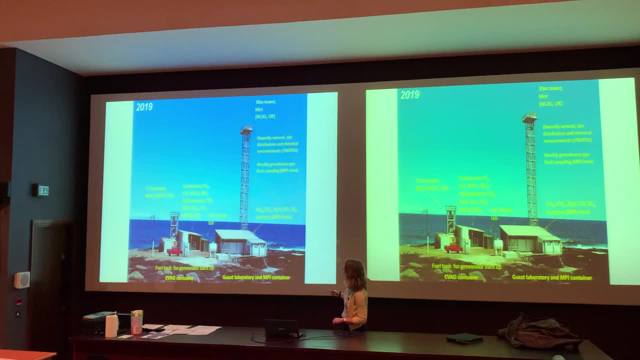 methane, all of these things. The German container, of course, looks better than ours, though we are updating ours as well. They're measuring greenhouse gases and all sorts of different isotopes. We've got this fantastic big tower that we can use to make our measurement. 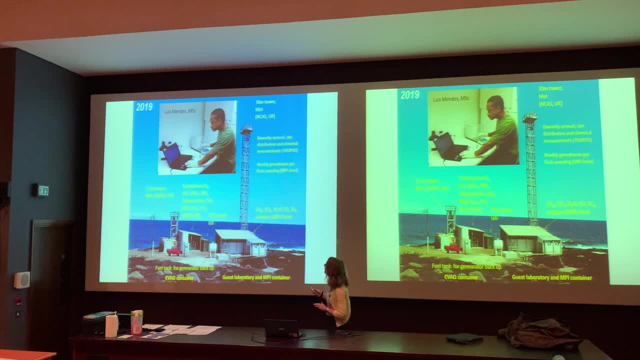 samples from as well. All of this is run extremely well by our experimental officer, Lewis Memphis, who is capable and lives on the island, And he's been working for us now for all of that time- for nearly 17 years- and does a great job and has other technicians. 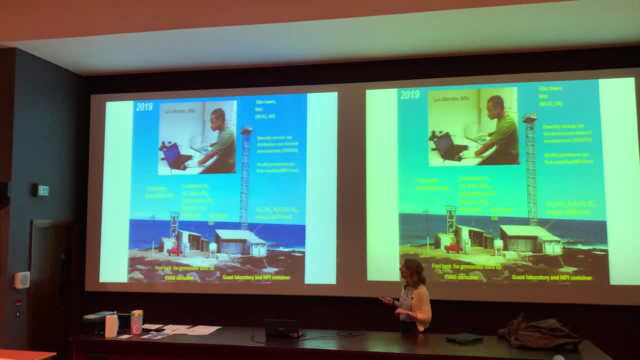 that work for him at the site as well. So they're pretty much there all of every day, which you have to be because there are lots of jobs to do to keep all of these things running And all the data is sent back on a nightly basis. 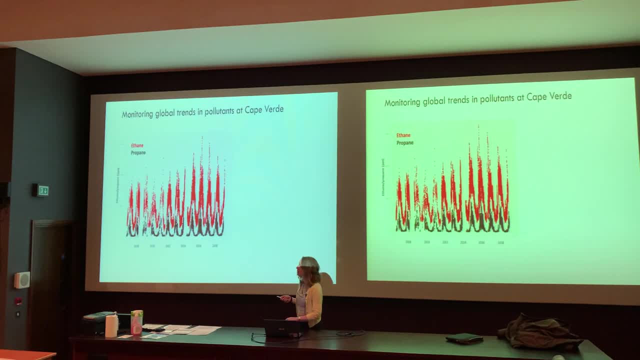 Back to the UK where we can analyse it. So one of the things we measure- or some of the things we measure at K13, we measure, as I say, VOCs, including gases like ethane, shown here in red, and propane, shown here in black. They're both things that are used. 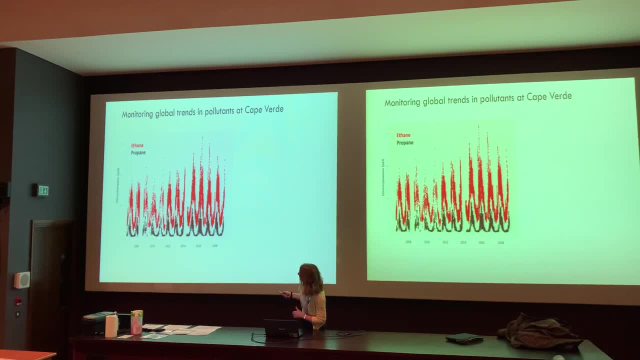 for natural gas. Now you can see from here, from when we started measuring in the round, the first thing to notice there are these big cycles, And this is essentially just a seasonal cycle. You see high concentrations in winter and lower concentrations in summer. This isn't really a big surprise. In summer, you have photochemistry that destroys the gas. Essentially, ethane reacts with the OH radical, and so you have these very reliable seasonal cycles. What's perhaps more interesting is how it's going up quite rapidly from around. 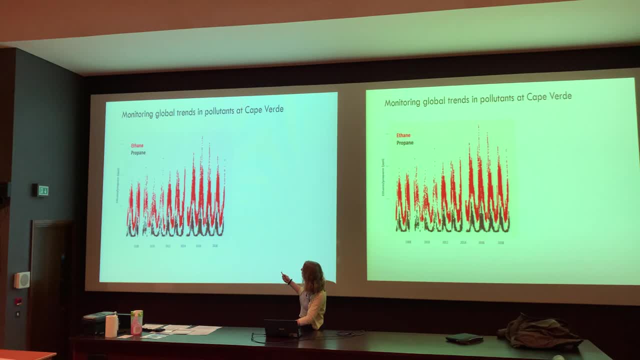 2009,, 2010,, particularly to around 2016,, and then levels off a little bit, but still is a lot higher than it was, And this is very interesting because up until that point, we didn't really know what was going to happen. So this is ethane in blue here, and this is. 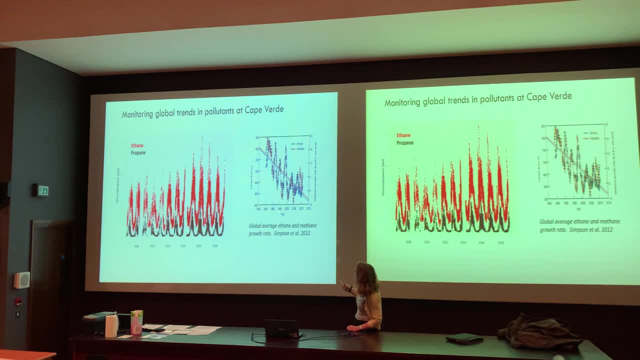 from around 1985 to around 2000.. So these are measurements from a paper published about 10 years ago, So essentially from the 1980s. for about 40 years ethane was declining in the atmosphere And you can see this really wherever you went, particularly in the modern 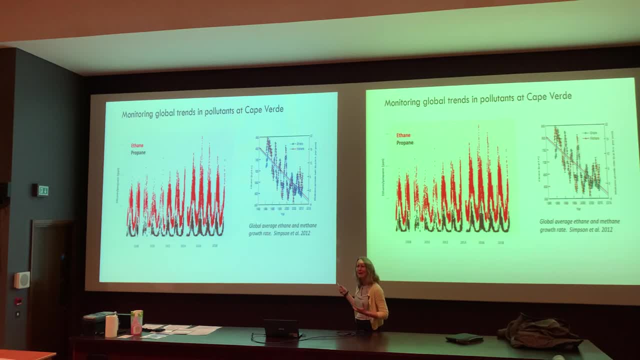 atmosphere, And that was due to, you know, clean air acts everywhere, people cleaning up their act when it came to fossil fuel combustion. Basically, this is a sign of success. So then we start measuring and thinking what's going on? We're starting to see it was not. 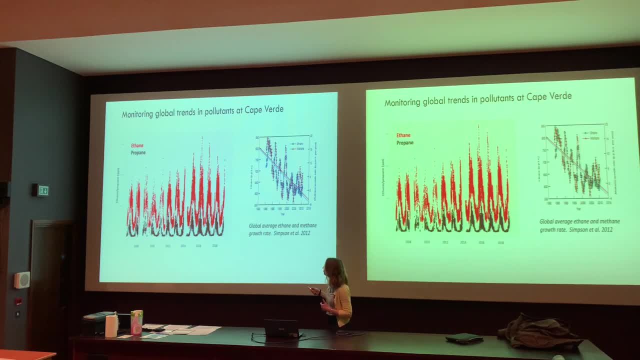 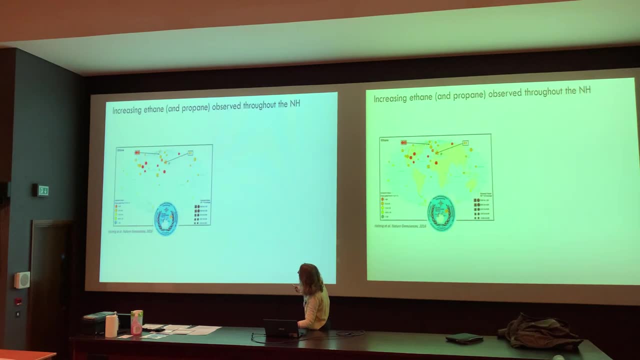 declining and then after a while it starts to go up and propane does a little bit as well. And then when we I told you you can't really see this very well, this is a map of the world, And each of these symbols here shows where we can compare with other stations. 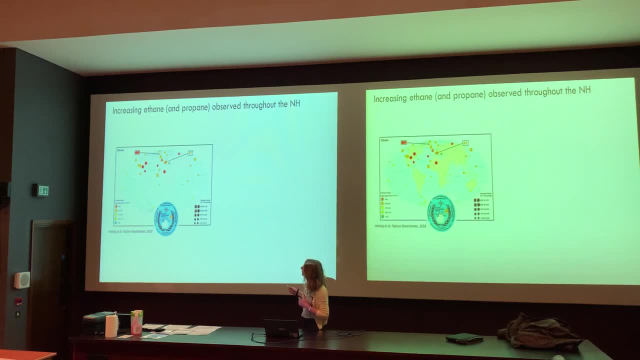 that are also measuring this gas And every time that the symbol is either red or orange, it shows where it's going. And then when we measure this gas, it shows where it's going And that shows that ethane is also going up over the same time period. The more red 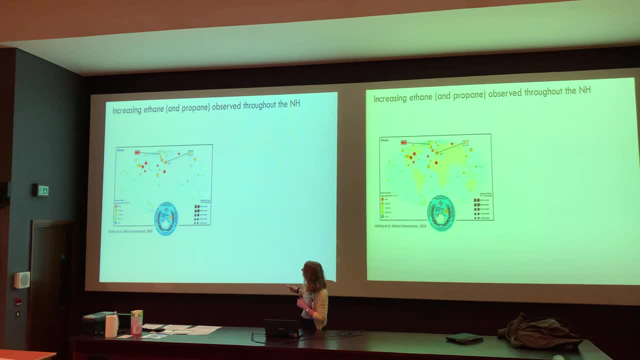 it is the higher that trend And the yellow shows where there's no trend and the yellow is all over the southern hemisphere. So basically what we introduced, A from the pattern of these emissions that were really pinpointed, most intense over parts of particularly. eastern the US and also from the nature of the time period of that trend, And then we really started to see the biggest increase between 2010 and 2015.. And from some other data taken in the US, we've basically attributed that to fracking and shale gas extraction. 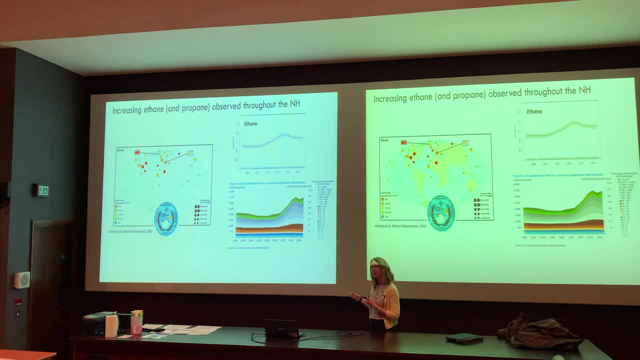 in the US, which is, I mean, they don't want to produce ethane. It is a byproduct of doing things in a way where there's bound to there's almost always a leaking of the gas that you can't control And that, so the trend in ethane really matches quite well. 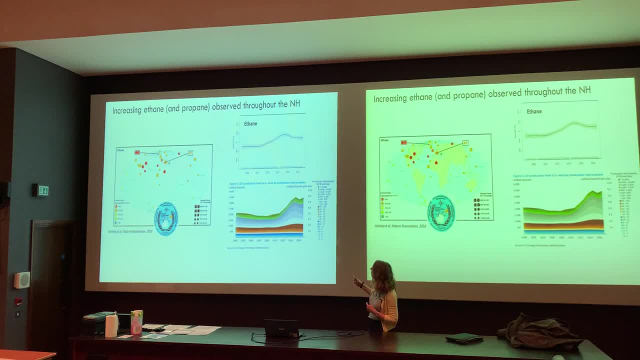 with the US production in terms of barrels of oil- a million barrels of oil a year- which is now somewhat stabilized, but I think could still carry on continuing going up because the capacity is there. It's only really the US that is doing this. A few years ago. 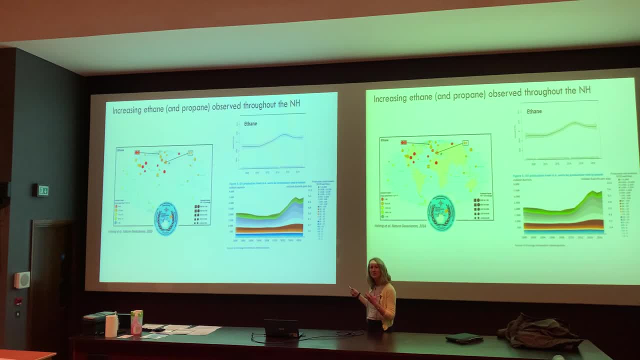 it was going to happen in the UK. There was a lot of talk about this. There was a little bit of earthquakes that were set off. The British public in the end did not have the right site for this, so it was effectively banned. So but what you know essentially? 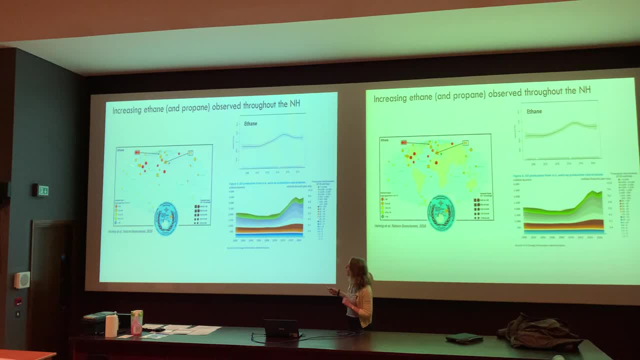 the bottom line there is that the energy extraction from one country filled up the entire Northern Hemisphere with ethane and reversed a 40-year previous decline in that gas. Oh yes. so what I would say is the increase that we see of ethane is not in itself dangerous to your. 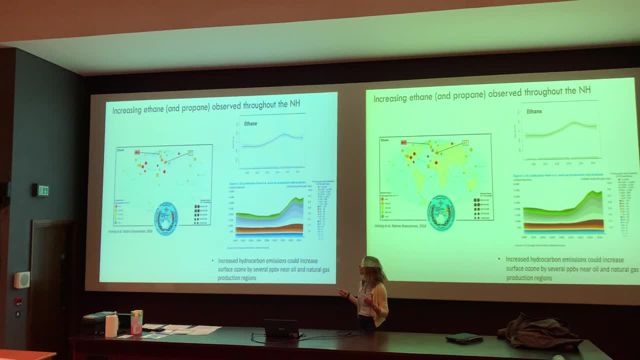 health. If you breathe a little bit more ethane, you end up with a little bit more gas. So ethane you won't have any ill effect. You're still talking, But maybe two ppb would be safe. But what it does do, alongside other emissions, is it increases surface ozone and 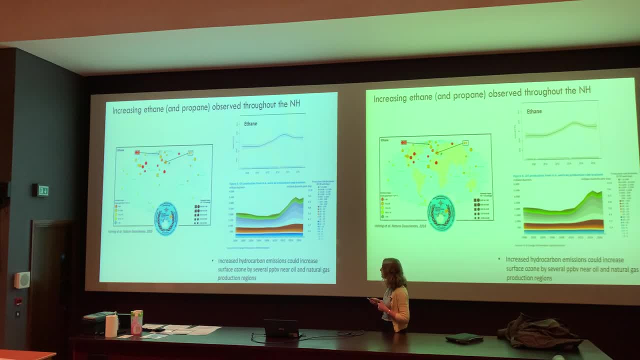 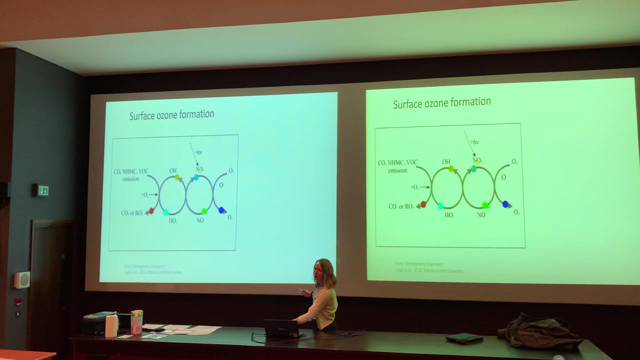 we've seen ozone as a pollutant by several ppb, certainly by near to the oil and natural gas production regions, And this is one reason why, you know, many US residents have protested against these emissions. Yes, sorry about this, I'm a bit head-on producing this cartoon. 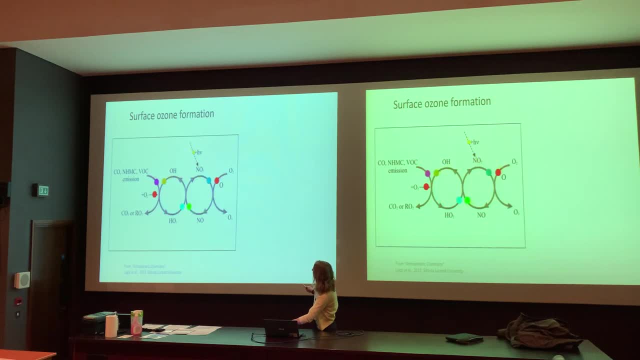 But it shows how ozone is formed. Ozone is a product here. Essentially, you need these volatile organic compounds like ethane and you need NO, which is mainly coming from things like cars, And this shows that the catalytic cycles involved in these gases in the end, convert oxygen to ozone, So ozone is spat out the other end And that's how you form it in the atmosphere And measuring this at different sites in Europe, how you can see how ozone has increased over the 20th century- at least doubled, maybe tripled over that. time, And that's due. it's stabilising more now in most places and that's mainly due over that time to the increase in global emissions that we've had. So we care about ozone. It's gone up an awful lot and we care about it because it's the second most harmful pollutant. 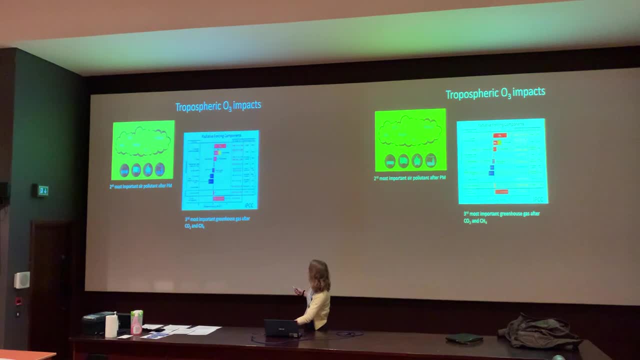 after particulate matter. I won't. I haven't got time to describe this in detail, but it's also the third most important greenhouse gas after CO2 and methane, after the carbon emissions, And we've forgotten, not really had much attention to that, but it does absorb. 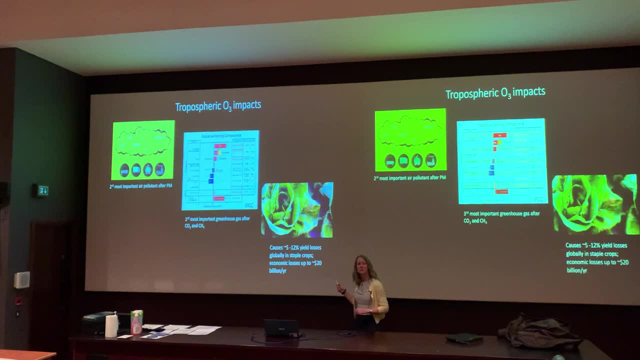 infrared radiation, And it also is damaging to crops. So there's, if you expose crops to too much ozone, you'll get this all sort of horrible damage, and that has a direct economic loss, of course, A really large one, particularly in places where ozone is large. 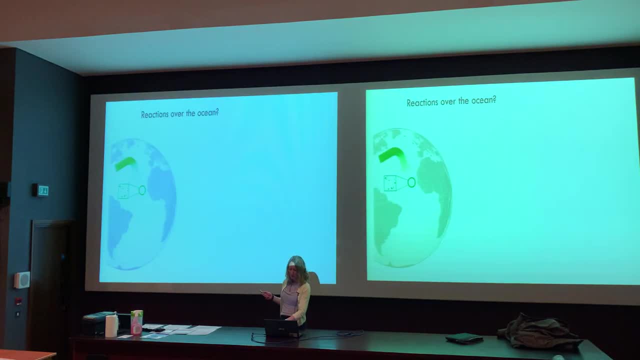 and a lot of crops are grown. So we ought to be- you know, we ought- to be aware of those sorts of impacts that are occurring on ozone Now. one of the reasons, another reason that we're going to Cape Verde is not just so that we can just sit there monitoring all. 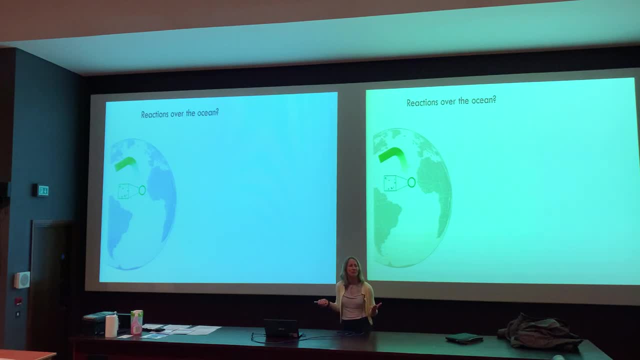 of these sort of pollutant trends and we have to wait 50 years, really, before we see anything interesting. There's also we can look at processes, And it's a really good place for looking at processes occurring over the ocean, because it's almost like being 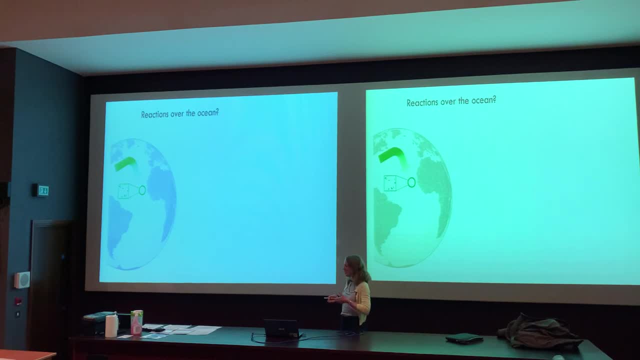 on a boat in the ocean because it's a volcanic island which shells really steeply into the sea and you don't have many coastal effects. There's no large seabed beds that can have like weird emissions or anything, So it's a really good place for looking at processes. 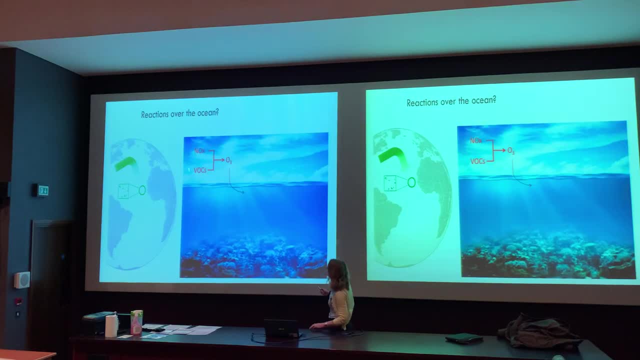 like this. Our main concern is: are there processes occurring over the ocean that we aren't really up-to-date or aware of? So you think we're in the UK. The ozone, for example, The ozone that we experience, that you're breathing in now, is really a function. 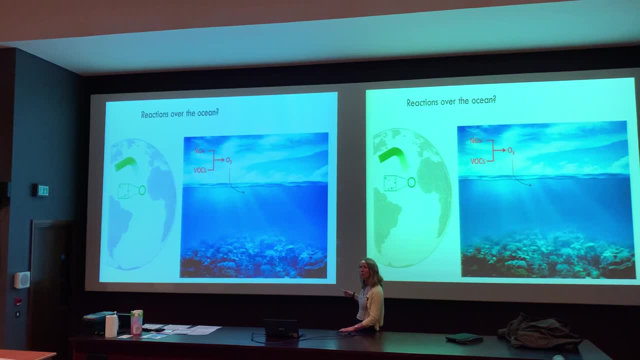 of what's been brought over by the prevailing winds, And that's normally coming from North America. So North America will uncertainty out by lots of the Butterworth emissions, make closed zones of the ocean, And of course there's the dioxide. Imagine these And you. 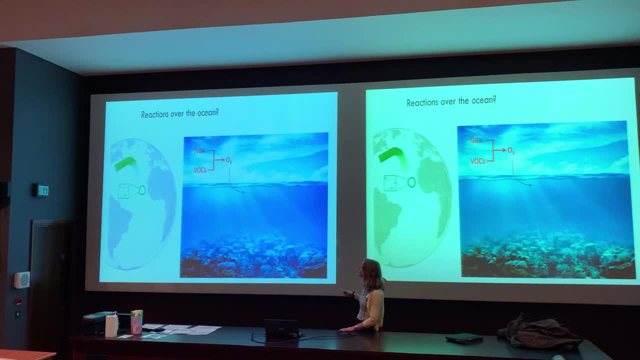 and that ozone will gradually decrease during its transport over the ocean, mainly through through two, through well, what we believe to be only two processes: definitions of the ocean and photolysis, so that the ozone in the breathing is a function of what has been brought to us from other countries and that what we're making locally as well for our 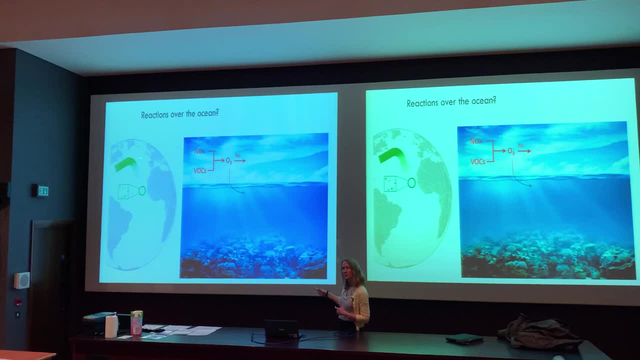 own lots of voc emissions because it has a life of many days, so it can survive transport over its continental, intercontinental time scales. what we were interested in was: what is there anything else going on? not not in terms of production, we know that pretty well, but in terms of what's. 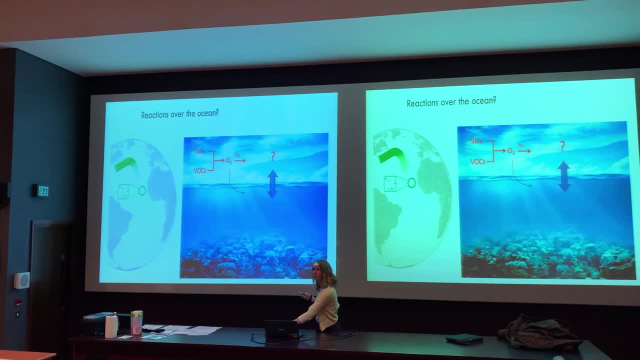 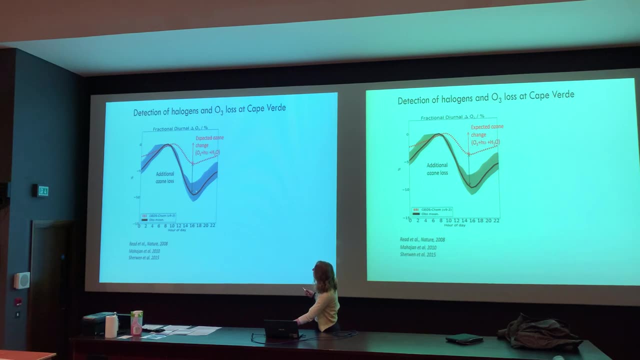 destroying ozone and the ocean. this, this ocean environment, is a perfect place to go to look at those processes. so, to cut a long story short, this is a typical cycle of ozone during the day, so you know the hours of the day here and this is just the percentage of its change from. 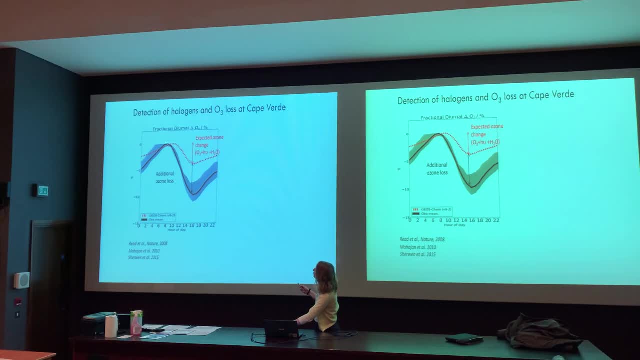 zero. so the point zero, whatever the ozone concentration is at about eight or nine am. and it's this part of the day that we're interested in because, unlike in cities where you would say you'd see just over an increase during the day, as it's formed from lots of eocs in very 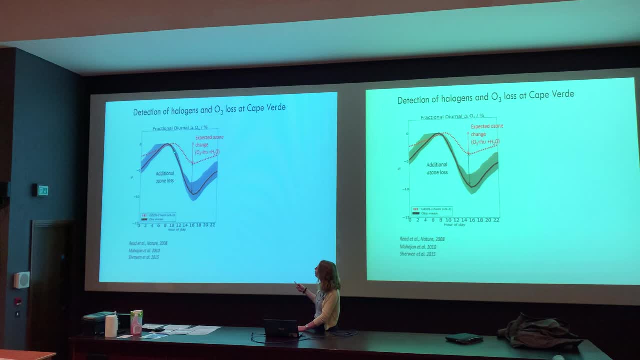 clean regions. what you're seeing here is this signature of ozone being destroyed. so we knew that there would be ozone loss over this region, because we know that this ozone photolysis takes place. but what we really was trying to see was that the ozone photolysis that takes place- and this is a process that's been- 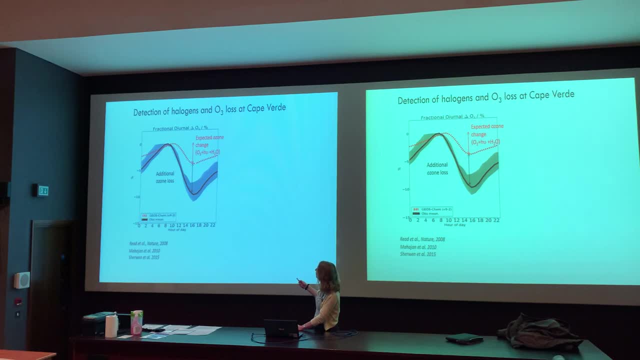 known for many, many decades as well, characterized, only really accounted for about half of the loss that we saw, um, and we were lucky that. so we, we had an idea that this was down to reactive hydrogen chemistry involving bromine and involving iodine, and we were lucky that a, uh, we basically 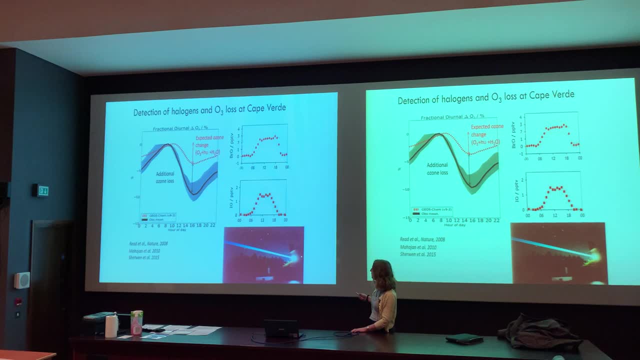 bought a lot of decay early, just for for a year, um an instrument from a colleague called john plane in the university of leeds. it's an optical telescope that essentially sends a beam around five kilometers away, balances it back and is able to make the absorption spectra of these gases. so 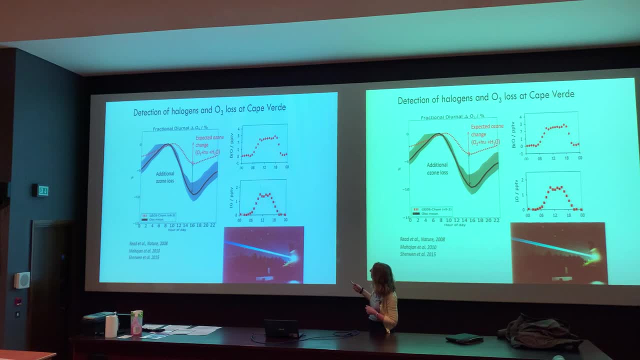 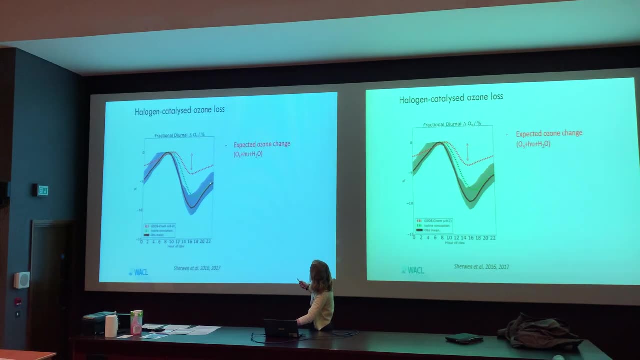 even though they're at very, very low levels- one to two ppt or up to three ppt there- and this instrument can measure them well- and even though these are very low levels, those levels could explain this full ozone cycle that we saw. this is really a new process that no one had thought of. 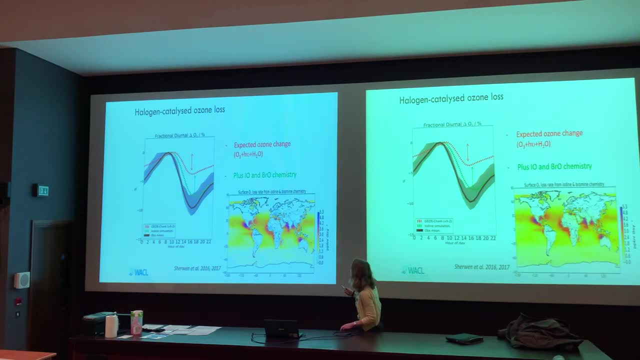 out before in these sort of open ocean regions and when you um do the calculations, put all this through a global model, um, essentially this is the extra ozone loss per day that you see due to this idea of breaking chemistry, and essentially it's losing an extra seven ppb per day of ozone in many. 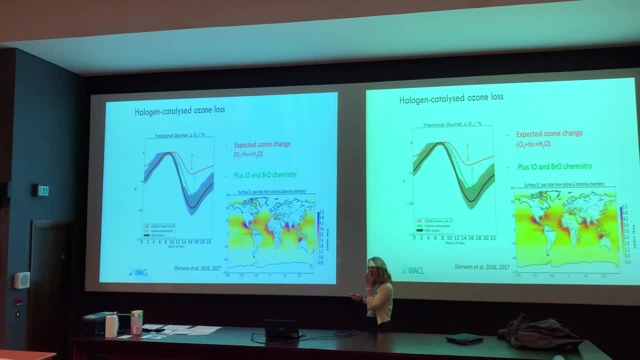 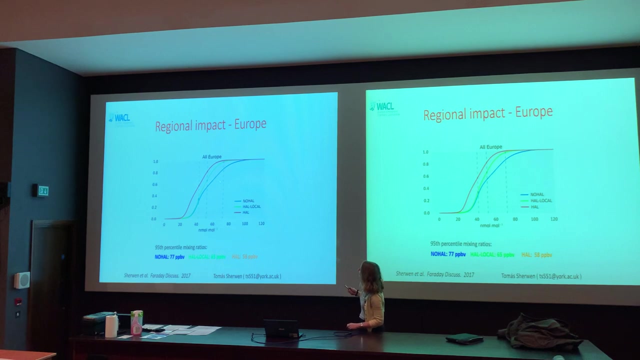 regions and that's really important from a health perspective, because the um, the world health organization limit, is around about 70 ppb. anything that we can do, anything that's done to reduce that level, is a good thing and we were calculating that um, even in cities- this is in london- um, the well it's. i'm not going to this. 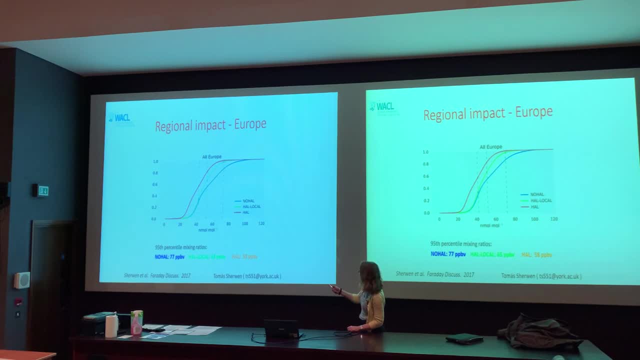 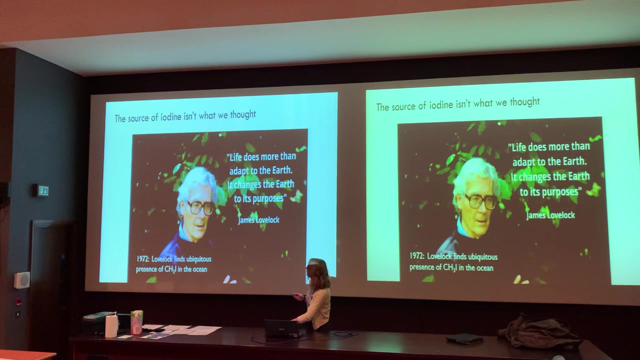 graph is quite complex, but even in london if you take 50 uh, it can reduce the ozone concentration by 10 to 20 ppb, even in regions that aren't over the ocean. the big thing that my research group did was really just think about how these halogens being sourced. we know that bromine. we knew pretty much that bromine. 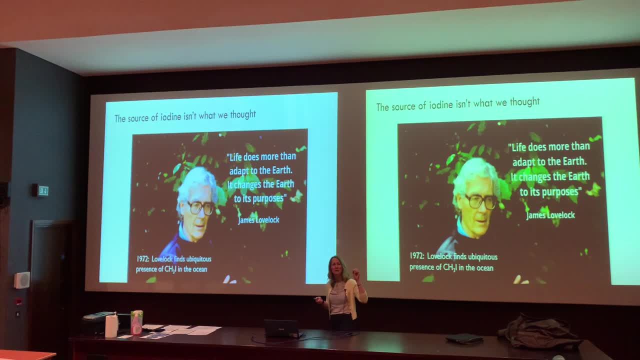 comes from sea spray. so the action of sea spray releases a little tiny broken enriched bromide, enriched droplets, into the air and that bromide ends up being released into the gas phase and that basically stimulates ozone loss. chemistry- at that point we only really knew about methyl iolite in. 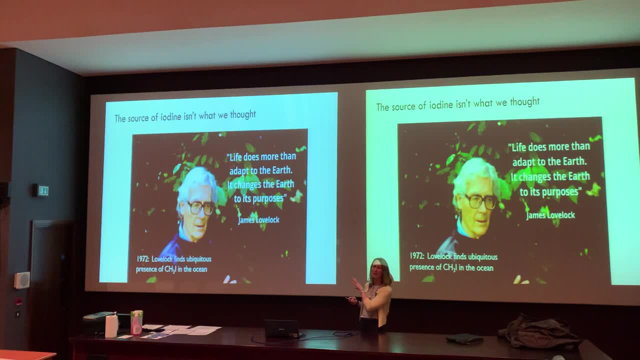 terms of the source of iodine. that came really from james lovelock's era, who in the 1970s did a whole bunch of research proofs and actually he brought iodine into his guy theory. people might be aware of the guy theory, which basically says that there is an altruistic reason to uh, the nature produces certain gases and iodine. 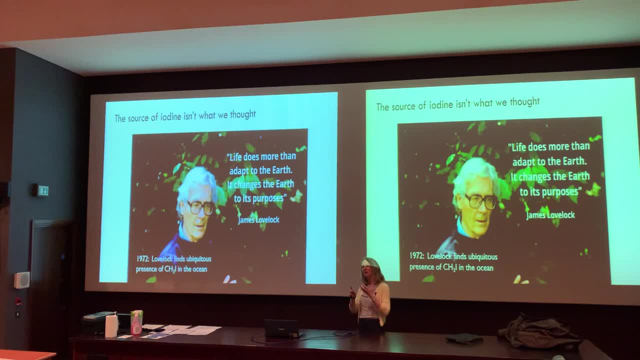 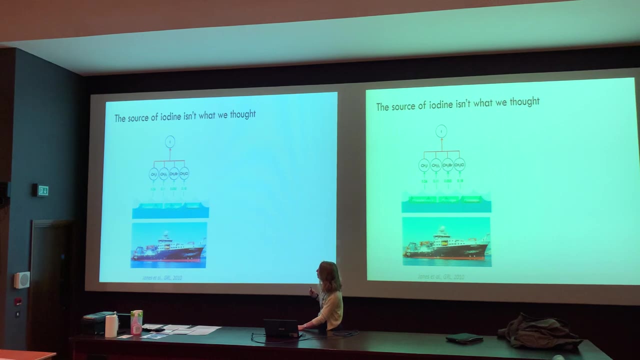 is actually a central nutrient for health. so his idea was the ocean was kind of altruistically providing iodine that could be transported to terrestrial regions. um, for health. anyway, we found by doing our own research we found that the iodine was not the only organic gas emitted by the ocean. you get some of these. 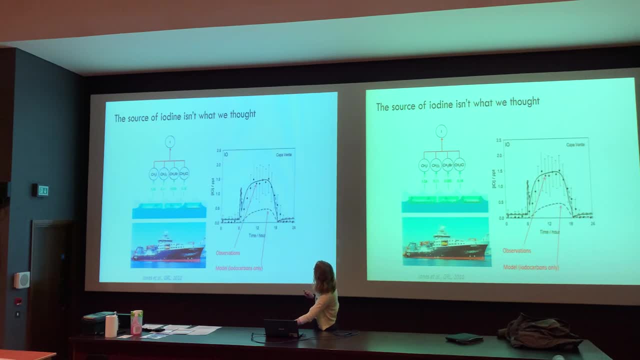 other exotic ones as well. but even those when you add them all up and you do some calculations, we're not able to explain the levels of iodine oxide, this io that we saw at k birdie. so you can see the levels of about one and a half ppt observed. these are the dots with the error bars. 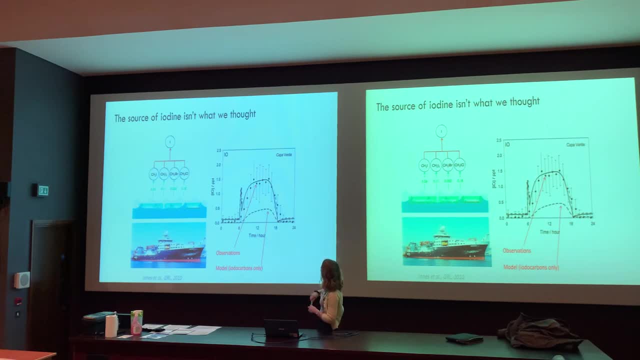 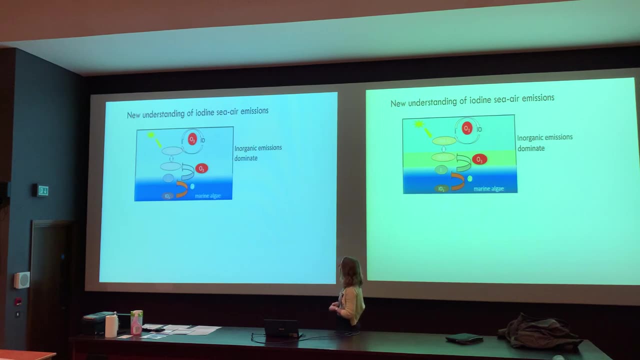 if you just include those organic compounds there, you only get up to this docket level lines of about a third of the way. what we discovered was it was actually chemistry occurring on the ocean that was giving rise to the dominant source of iodine. so we discovered: 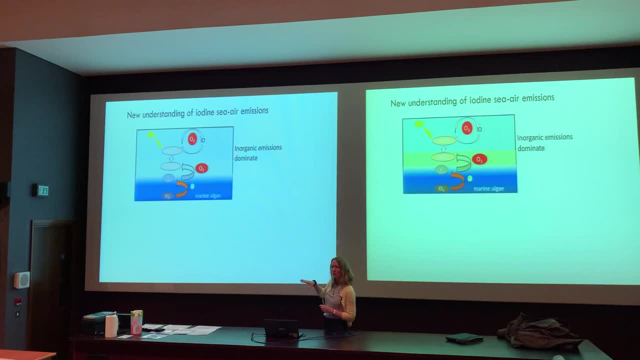 its ozone itself reacting with iodide, which is naturally present along with other salts in seawater, and that ends up, through very complex chemistry, giving rise to a gas called hri, and also to molecular iron into i2, and that turns out to be what we think about 80. 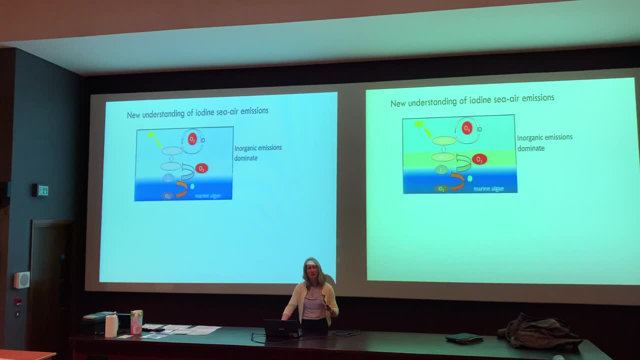 of the total iodine source. so it's a totally different way, because the mix of another organic gases are mostly produced by biology in the oceans. this is really just a chemical source, and if you put that source then into the model, you then come up with a solid line, which is the model. 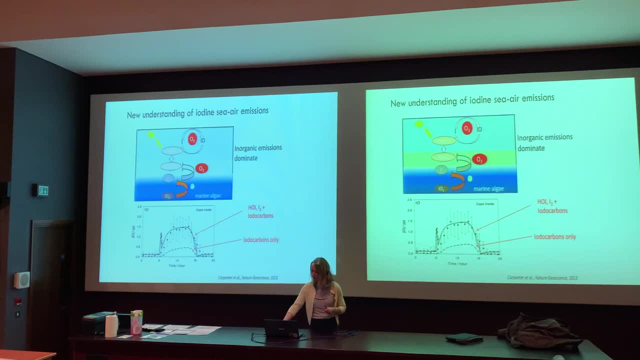 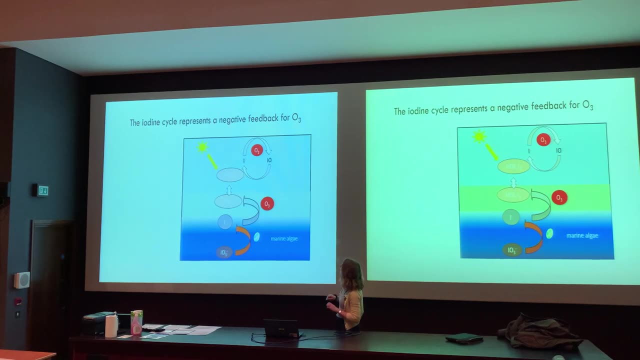 with all of these gases in which does seem to explain the observations. i've only got two or three, two slides left. i think what's interesting about the cycle is it's a negative feedback, because the more ozone you have, the more iodine you're going to get being emitted from the ocean, because ozone is a driver. 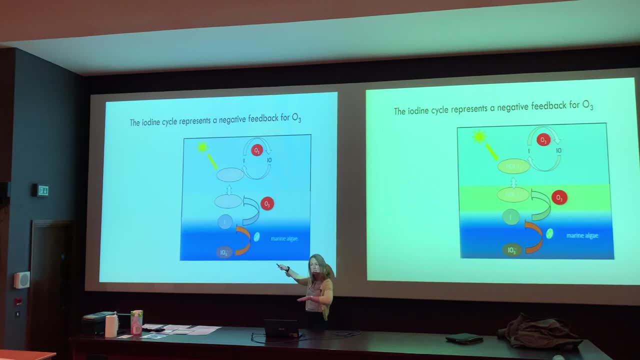 to basically convert that iodide which is in the seawater from dissolved phase and to make it into a gaseous phase. so the more ozone you put in, the more iodine you get out. but the more iodine you get out, the more you destroy ozone because you get cycles very similar to sort of stratospheric. 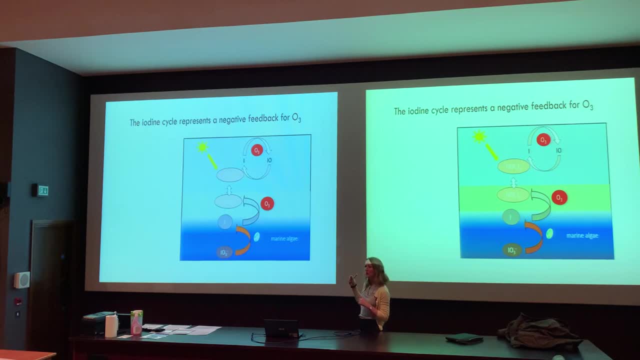 collagen chemistry which destroy that ozone. so it's a negative feedback cycle. and, interestingly, you've seen the plot i showed before where ozone has increased over the 20th century due to pollution. well, we surmised it, that was the case. there should be more iodine now than there was in the past because the ozone should have basically stimulated the 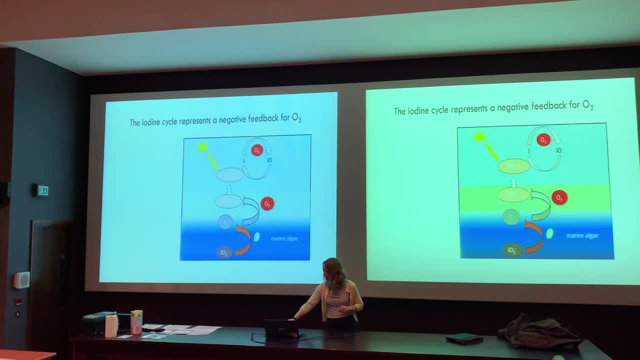 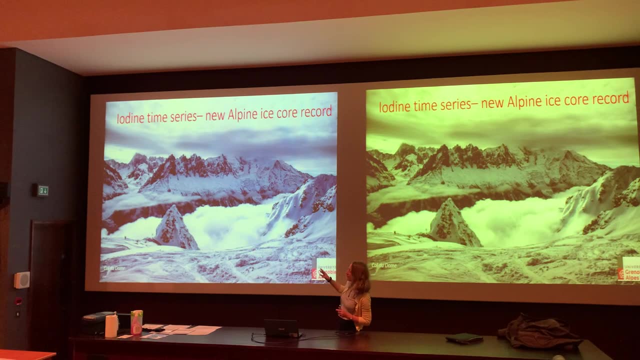 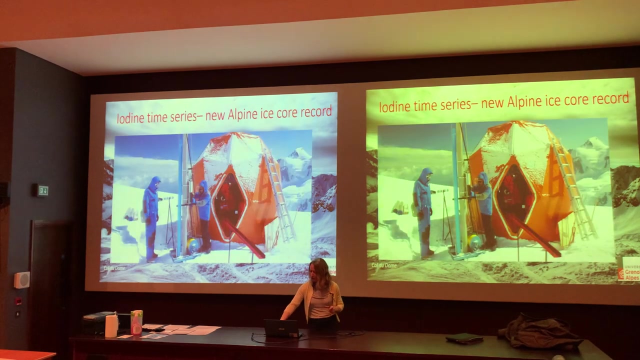 iodine to come out of the atmosphere, and that was just a theory until about three years ago, where we were contacted by the university at removal that had extracted some ice cores from um. basically come with a helicopter and they drill down several hundred metres into the. 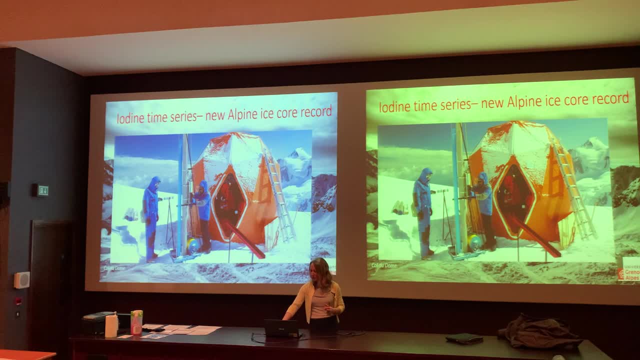 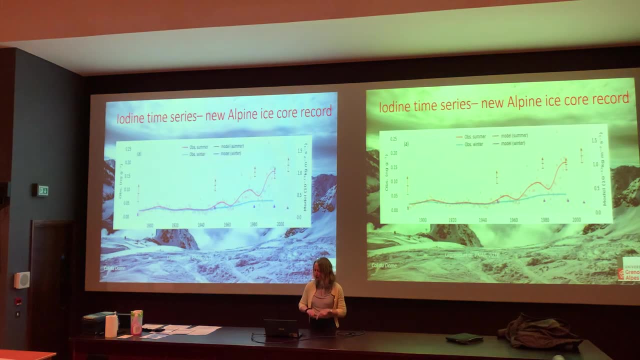 ice and extract an ice core. they take that back to the lab and they work from there. that ice core enables them to go back, certainly not millions of years, but a couple of hundred years, and they went back to basically the very late 19th century and the rest of the 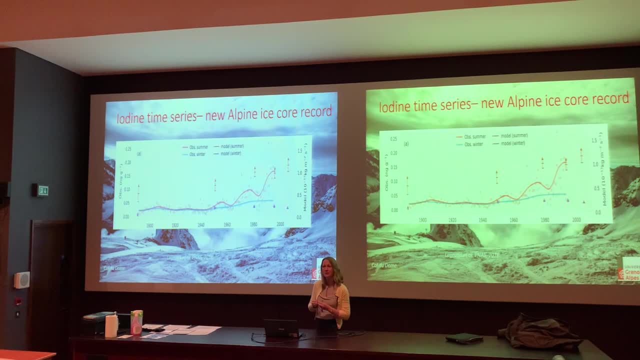 circles is their observations of iodine in that ice that they reconstructed into a time series: the red is in summer and the blue is their wintertime. is the observations of winter. you can separate by cores whether it's a summertime, whether it's linked back. 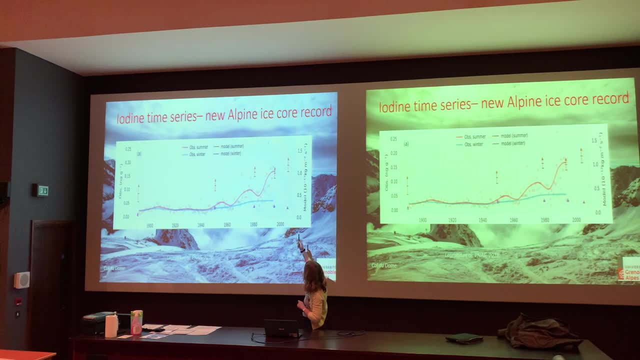 to summertime or linked back to wintertime, and you can see that. so essentially, iodine in summertime has nearly tripled from what it was in the early 1900s. the bars there, the arrows, there are our model predictions and they don't match it quite. 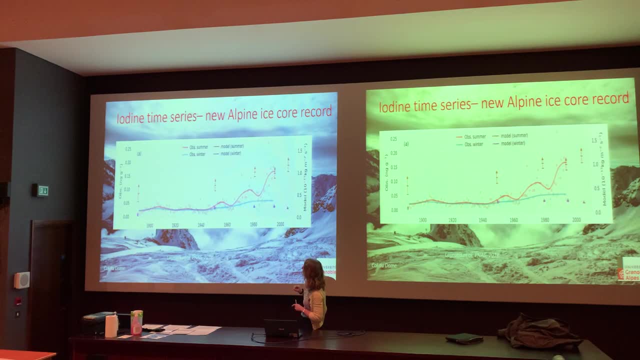 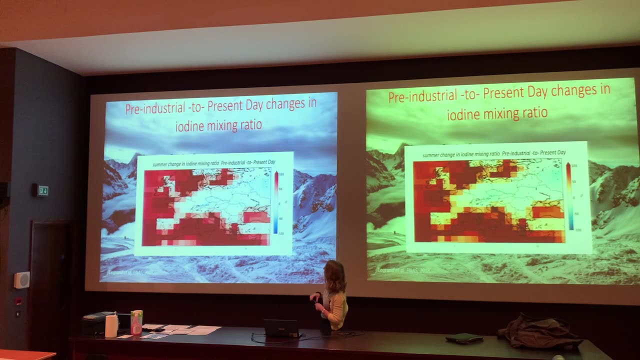 very perfectly, but they do show this difference in summer and winter and that they show that increase is compatible with an increase in emissions of iodine from what we think was going on in the pre-industrial era, so in the 1800s, to what it is to the present day. 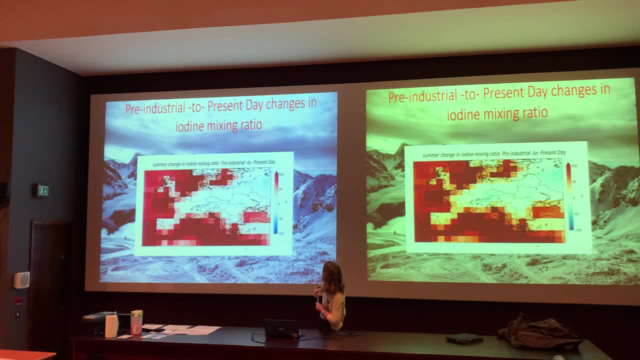 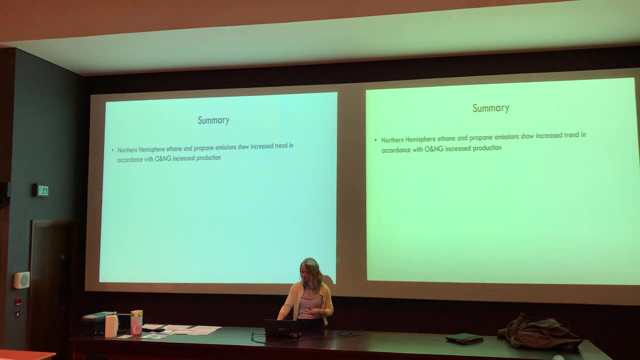 where that bar on the right shows that iodine emissions have basically doubled, gone up by 100%. so it was really nice observational confirmation that these predictions we have from from these iodine emissions was actually occurring and we can pick that up. so just to summarise, 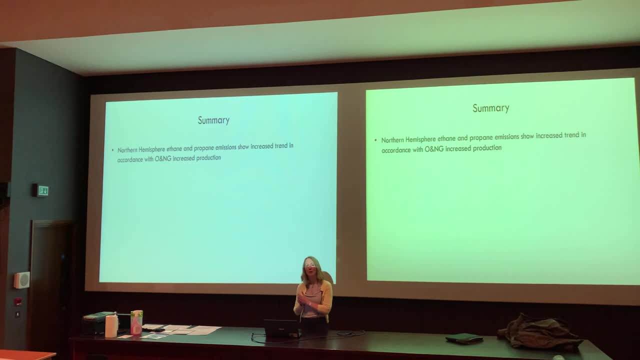 then. so I've started with the second part of the talk, talking about ethane emissions, ethane and propane and showing that it really felt really like a normal hemisphere and we were seeing this increased trend which seems to be in importance with oil and natural gas. 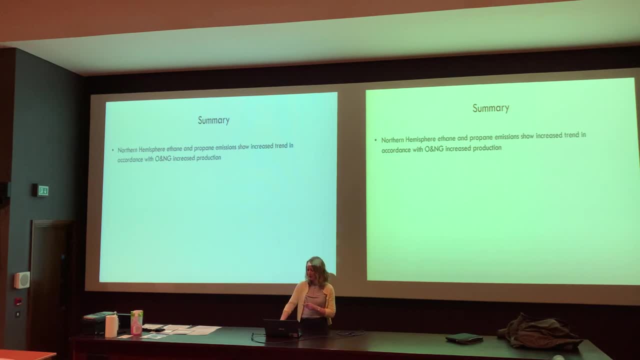 extraction stabilised a bit. now we'll have to see what that does in the future. and then we moved on to the clean atmosphere, thinking about the chemistry that occurs over the oceans, and showed you that this reactive halogen chemistry, which is a natural chemistry- iodine and bromide have been there.